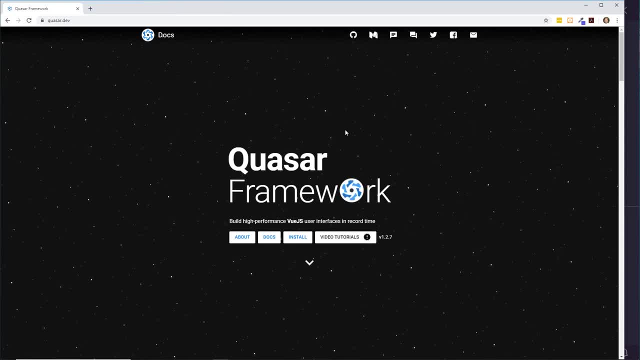 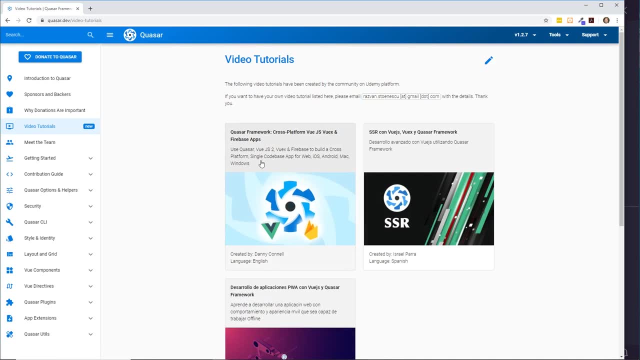 this framework over, do a tutorial on it. There's a lot of interest out there, So, which is cool. they actually do have a few video tutorials right on their homepage, So if you go to Quasardev, they already have a few up. I haven't watched them. Two of them are in Spanish and one of 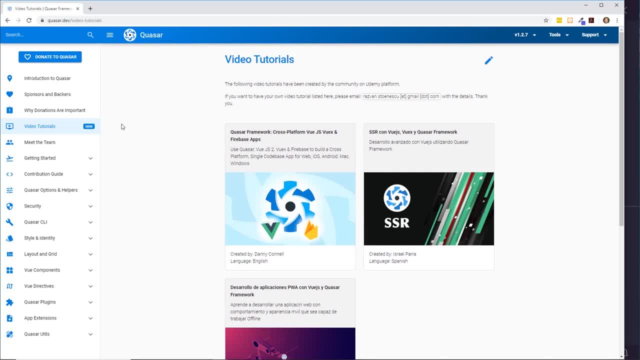 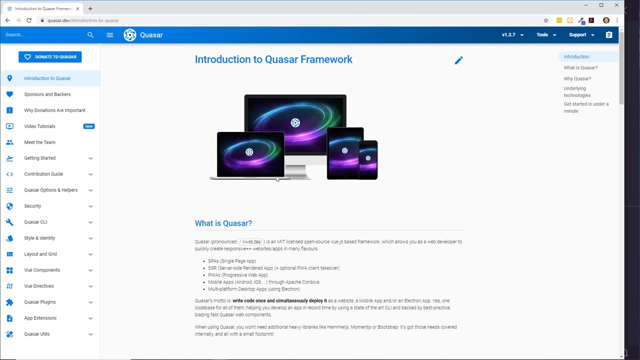 them is in English. So there's that Now, if you don't know what Quasar is, they describe it in the introduction to Quasar as a MIT licensed, open source Vuejs based framework which allows a web developer to quickly create responsive plus plus websites. And what's cool about Quasar? and you know? 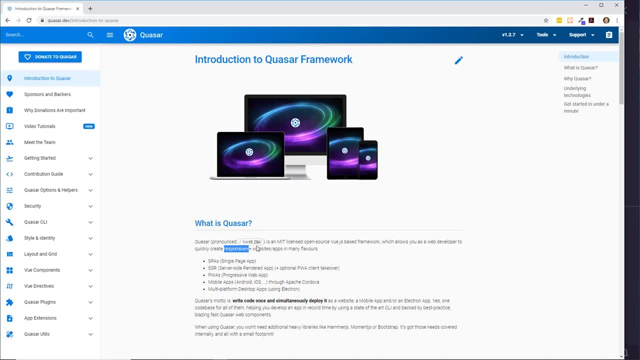 different than like Vue to find and other like material design type frameworks is this has a lot of cool features: to create one app but then be able to deploy it as a single application. So if you don't know what Quasar is, they describe it in the introduction. 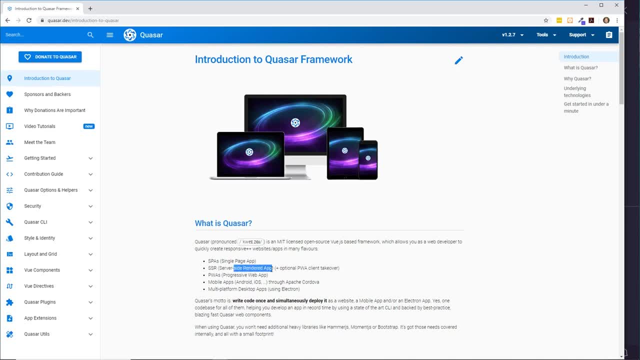 to Quasardev. So if you don't know what Quasar is, they describe it in the introduction to Quasardev. So if you don't know what Quasar is, they describe it in the introduction page. app as a server side rendered app: SSR. So you guys are probably familiar with Nuxt. 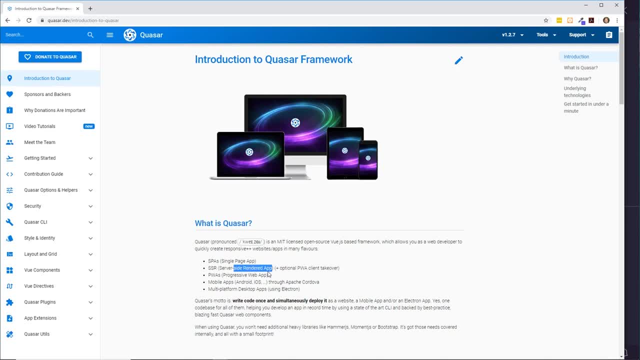 things like that, Like Nuxt, like those server side rendering or next, But this one has a built in. you can also deploy it as a PWA right out the box And something that you don't see too often. you can create mobile apps out of it and also electron apps. So 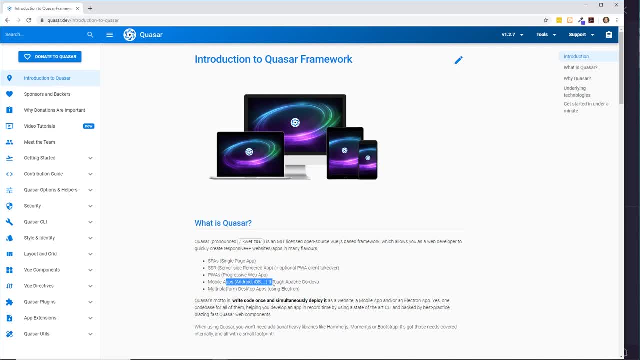 you can create like basically desktop apps and mobile apps, and it's really easy to do And you don't have to install a ton of plugins. So to get started, you can look here. There's actually three different ways you can get started with Quasar. 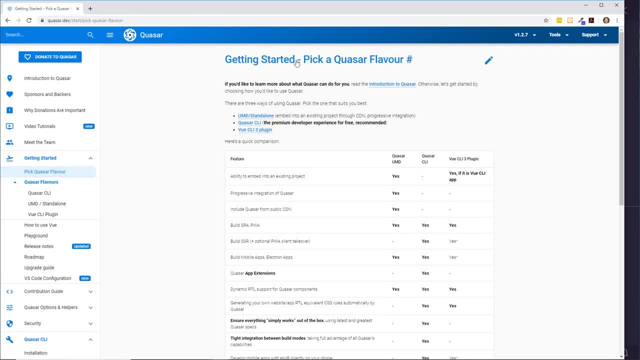 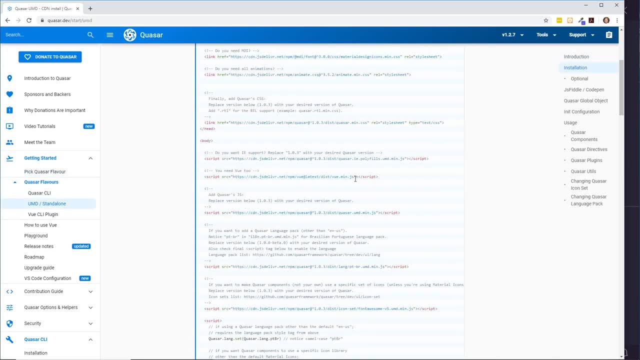 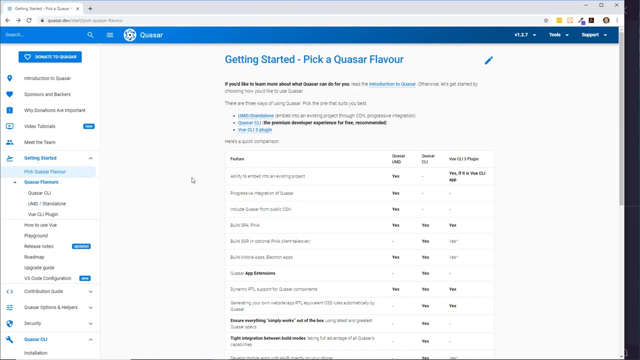 And they actually have a little handy-dandy getting started guide here. So you can either kind of just use it as like a script tag inside an app already- And you can certainly do that Sort of like- you can just throw a Vuejs tag in any sort of HTML file and add Vue to your app, to your website. 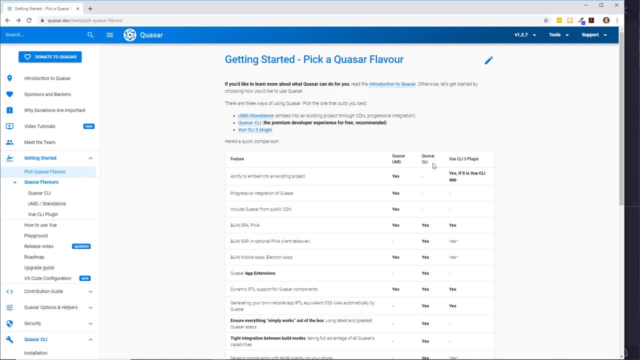 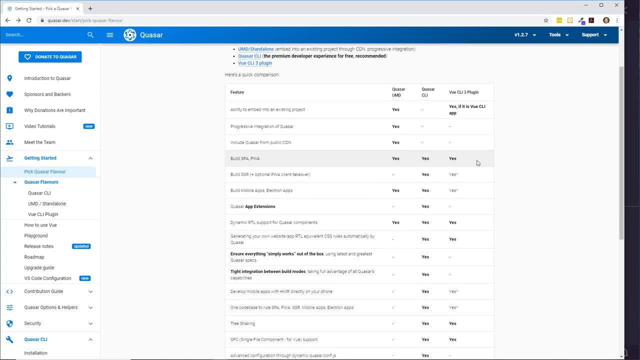 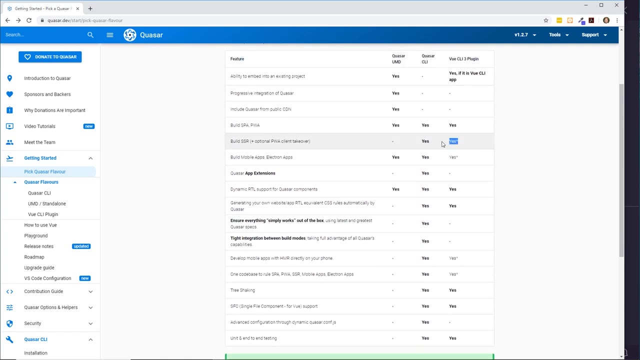 You can also use the Quasar CLI, which I'm going to show you guys later how to use, And then you can also use Vue CLI 3 plugin. So it seems like there are some advantages and disadvantages of all three of these. Like, for example, Vue CLI 3 plugin. it says you can build SSR and Electron apps. 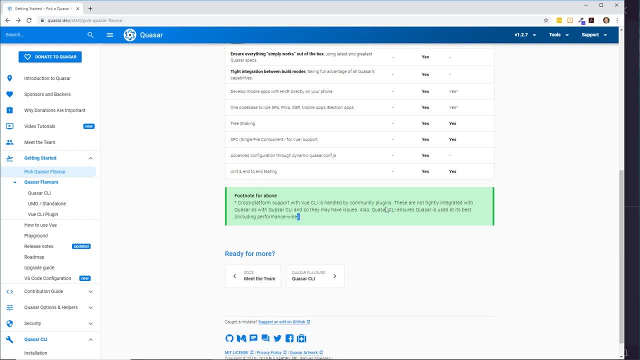 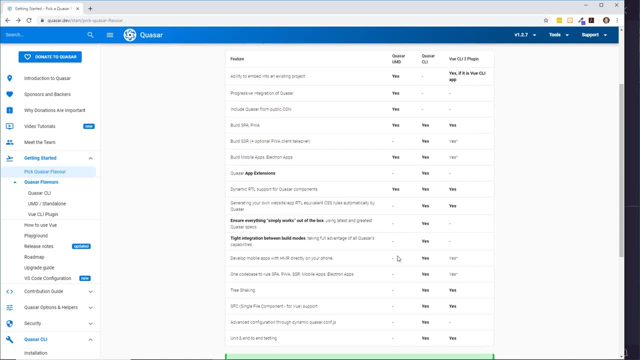 But there's a little star next to it And if you read this, it says that they're not tightly integrated with Quasar as much as the Quasar CLI, And so you may have some issues. So that kind of makes me think that if I really wanted the full features of Quasar, I probably should just use the CLI. 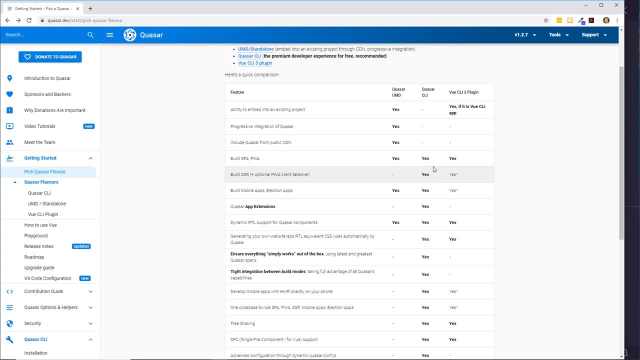 And the CLI is like. basically using the Vue CLI, You create everything using the CLI And it sets everything up for you And it has some powerful features And it has ways you can quickly get your Electron app up and running Or create a SPA up and running. 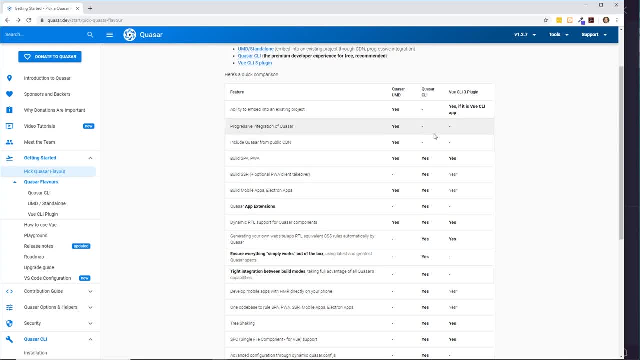 Or create a SSR version up and running or PWA. So I think that's the best way to go If you're just looking to use some of the other cool like Quasar components, sort of like- if you're going to use it more like using Vue Defy. 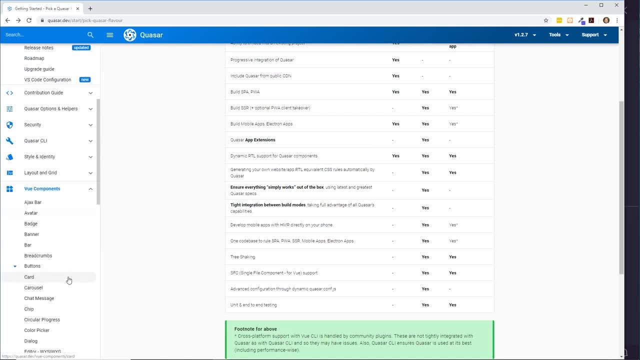 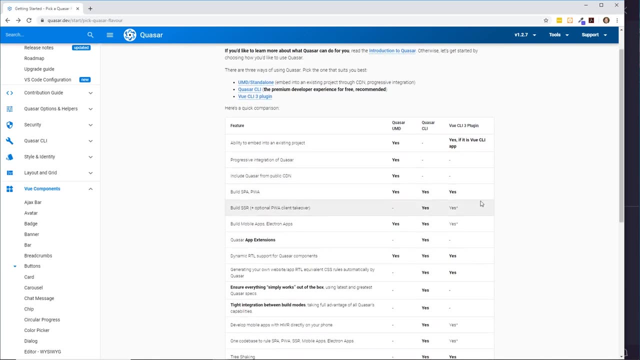 So you're just looking at the neat layout and grids and the Vue components, Then you know it's probably fine to use the Vue CLI with the plugins, But it looks like if you want the full power, the Quasar CLI is the way to go. 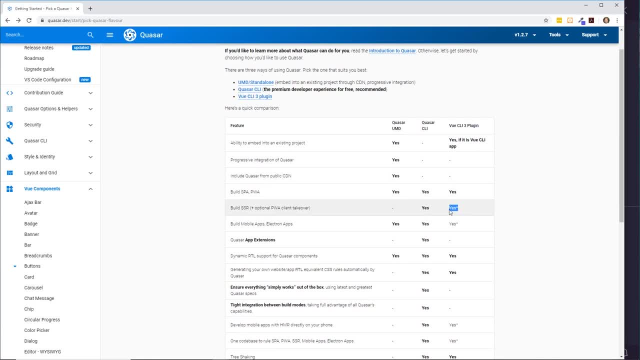 Although I mean if you've used Quasar. I'd love to hear If anybody's used Quasar, leave a comment below, Let me know how you guys liked it And if you ran into any problems using it, And if you've used it with Vue CLI or did use the Quasar CLI. 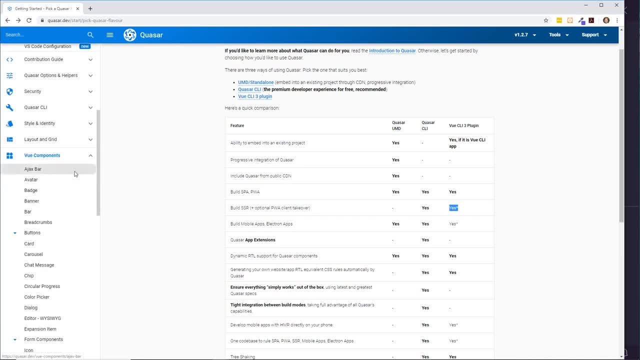 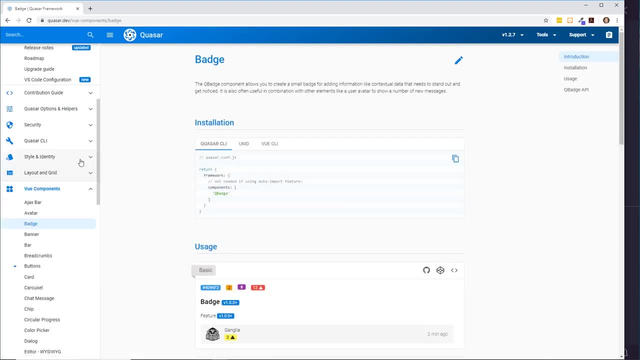 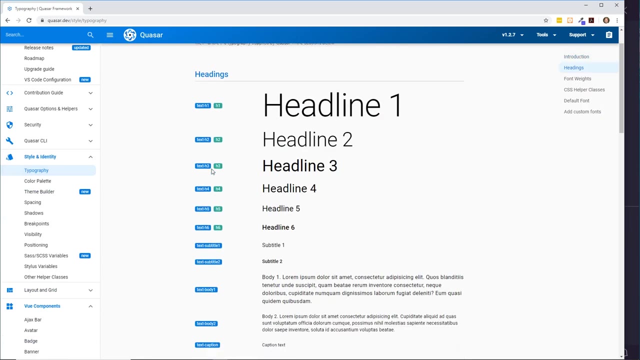 I'd love to hear that. So you see, here there's tons of different components that come built into it, Like carousels, banners, badges. It also has its own, A bunch Of its CSS type CSS tags classes that are built in that you can use. 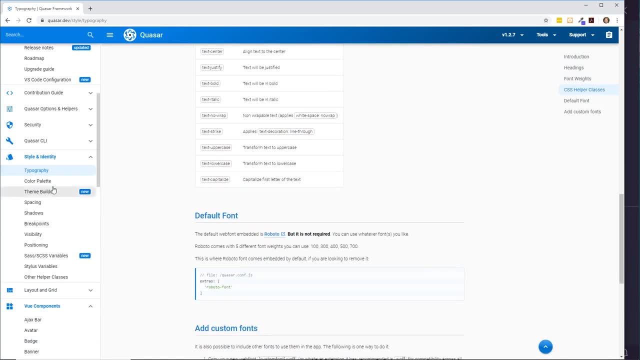 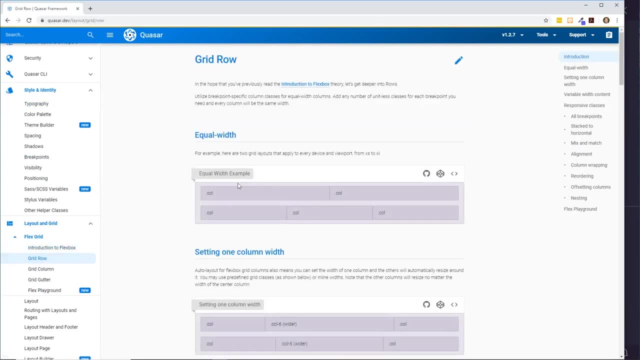 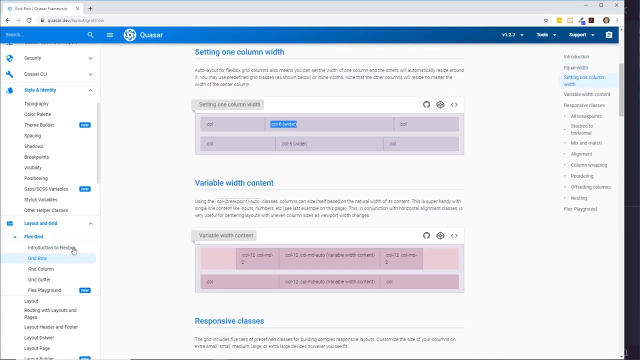 It sort of feels like using Tailwind. that way, You can actually do your whole layout. It's has flex course built in So you can use like column. just put col as your class names And you can really easily create your own columns. 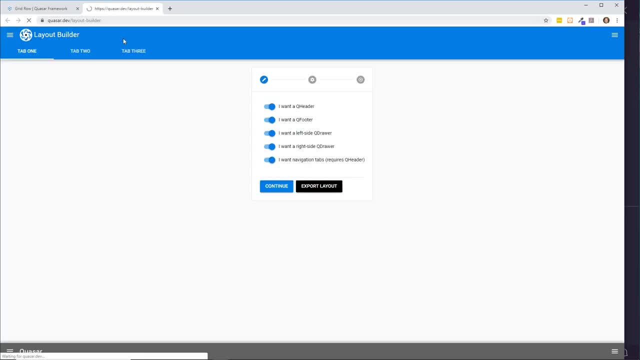 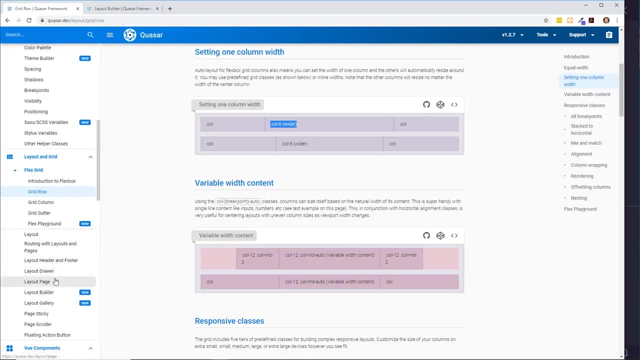 And then they have a layout builder. If you even want to create your whole layout here and then export it out, which I think is funny. There's just tons of different layouts and grids, And we'll take a look at it a little bit of that. 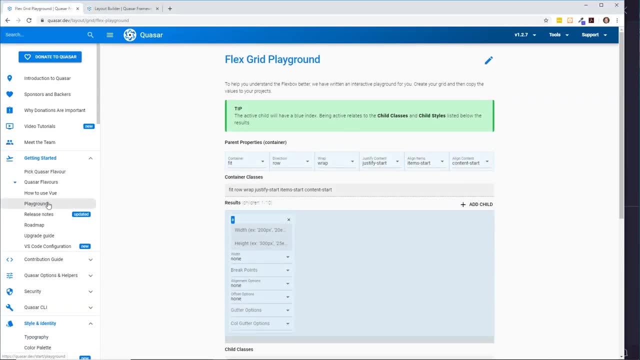 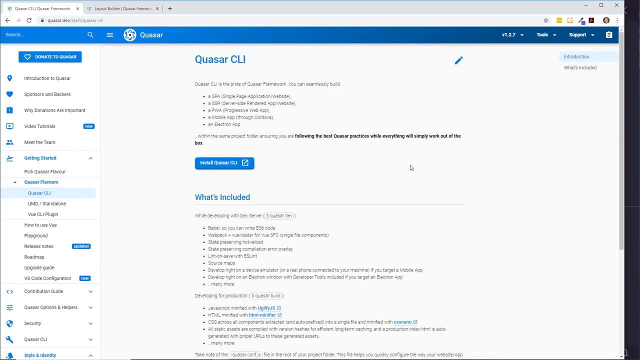 So let's start with this view, the Quasar CLI, which I think is probably the easiest way to go, And what I'm going to do in this demo is we're just going to kind of get used to installing Quasar, kind of taking a look at some of the components, but I'm really want to make this. 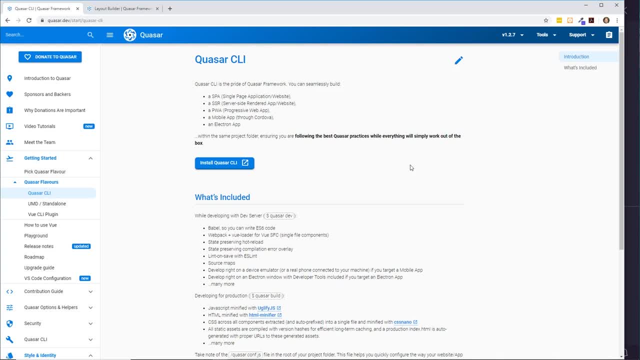 A multi series, multiple videos. I need your help with what video I should do next. So this will be a sort of an introduction, but if you guys really like this, I want to make another video and we're going to deep dive into into more of this. 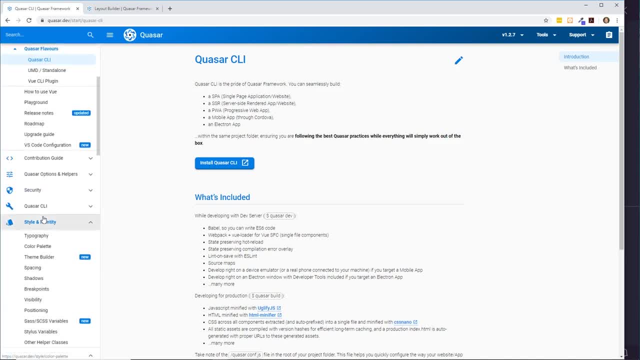 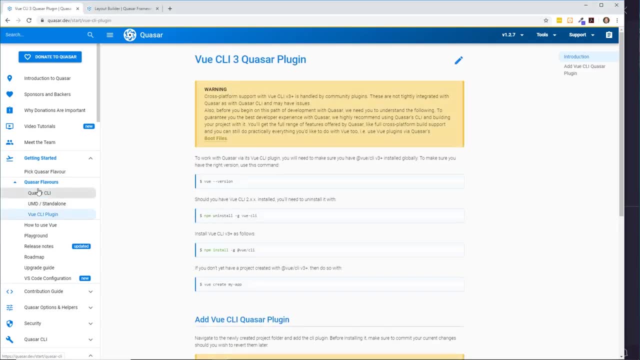 Cause there's there's so much to Quasar like this. this video could easily be like three hours long, but I want to keep it much, much shorter for you guys. So to install the CLI, it's if you go to the getting started. 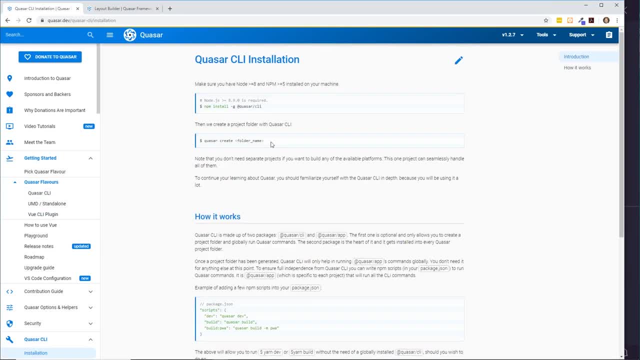 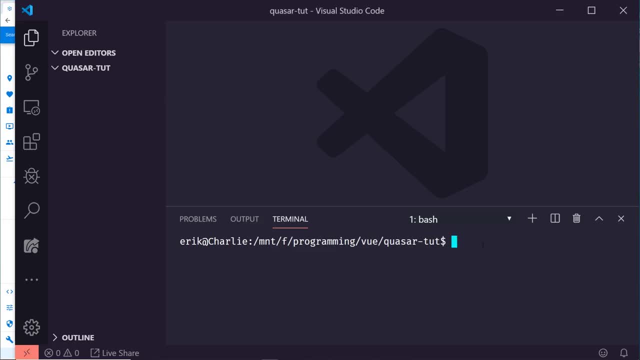 Okay. So if you go to getting started Quasar CLI and you just need to use NPM, install tack G, Quasar CLI, So something like this- my keyboard's a little quick clicky, So I apologize in advance- NPM salt, tack G and then Quasar CLI, like that, and that'll install it. 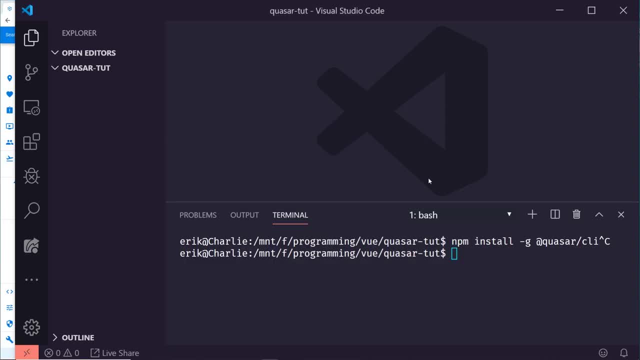 And then you can use Quasar crate and create a project. So let's go ahead and do that. So I have visual studio code open here and just have the open terminal. So Quasar crate, I'm Quasar demo. You can see here. it'll open up this installer here. 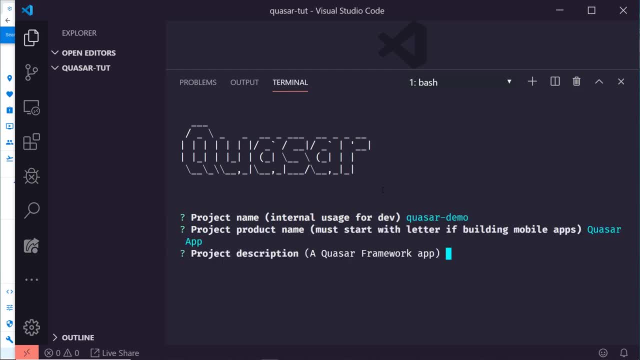 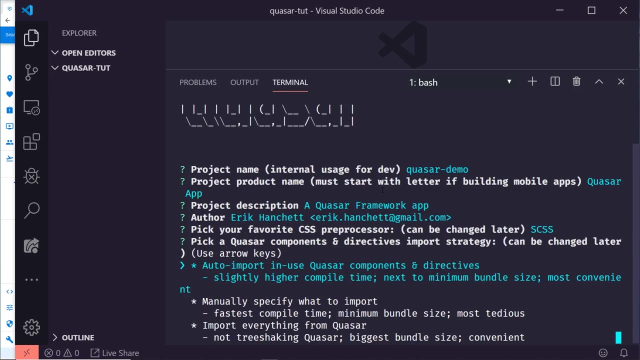 And it's going to ask us a few questions Like: what do you want to call it? Demo, um project description? author. Of course it's me. You can choose between SAS and SAS with CSS or stylus- And I know um, this is fine as CSS- and then you can auto import and use Quasar components and directories. 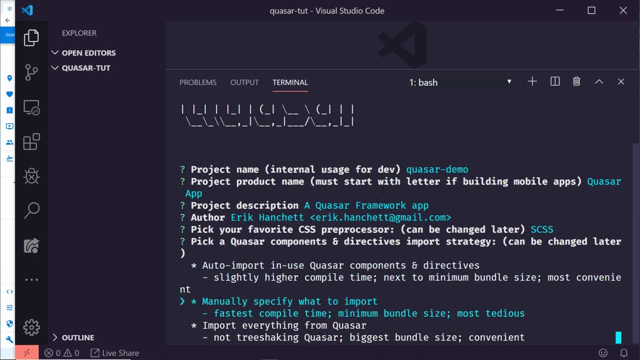 Slightly higher compile time. next, to minimize bundle size Most convenient. many manually specifies what to import. uh, import everything, So I I just take the recommended one: auto import in using Quasar components and directives. You can do that inside the configuration file. 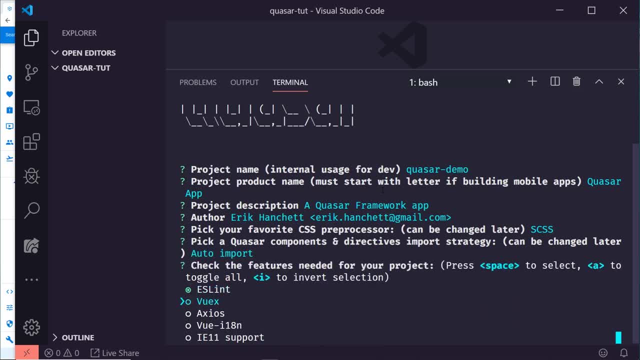 I'll show you guys how to do that. And then it asks you what features I mean. this looks pretty similar to view CLI three. Do I want ESLin, view X? I don't know, Maybe I'll do view X and Axios. 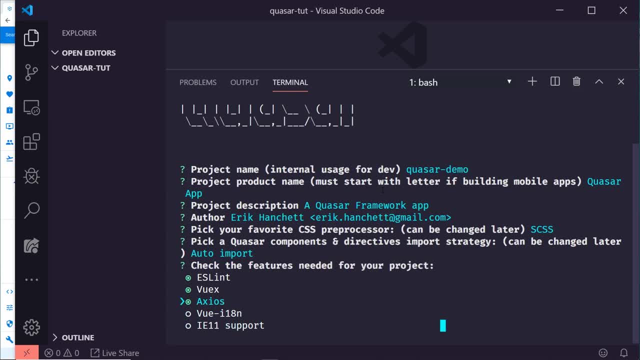 I'll leave off IE 11 support for now and internationalization And ask me What kind of ESLin preset presets I like? I don't know, I like prettier, some set that and this is kind of neat. You can actually create Cordova apps through Quasar. 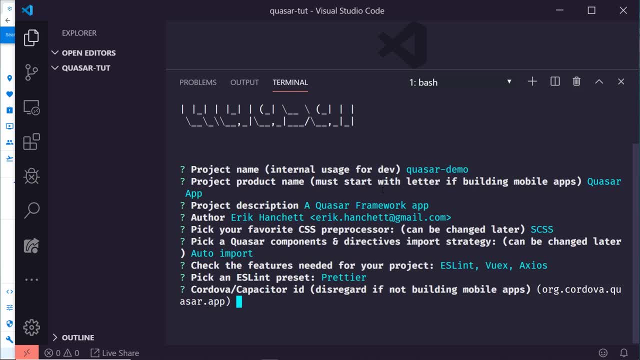 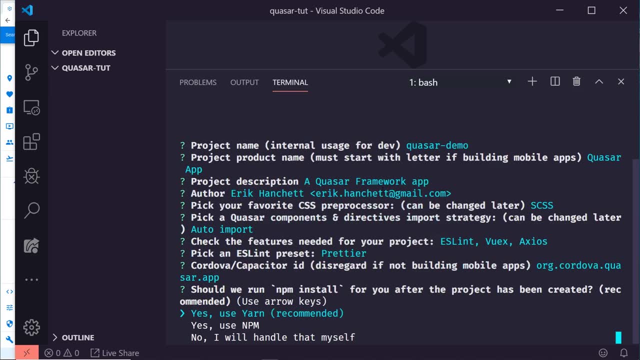 And it even asks you when you build it, like: what do you want? Uh, the capacitor ID to be. I'm just gonna leave it default for now. And then it asks you: do you want to use yarn NPM, or I'll handle that myself. 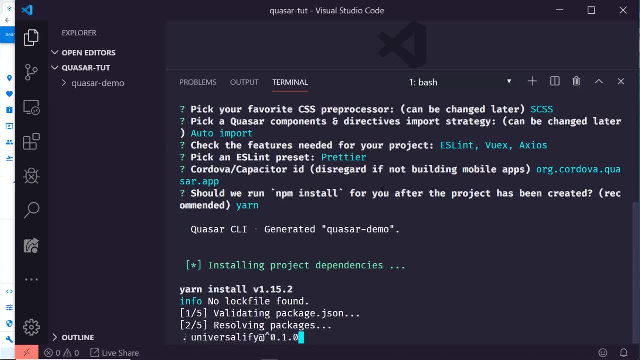 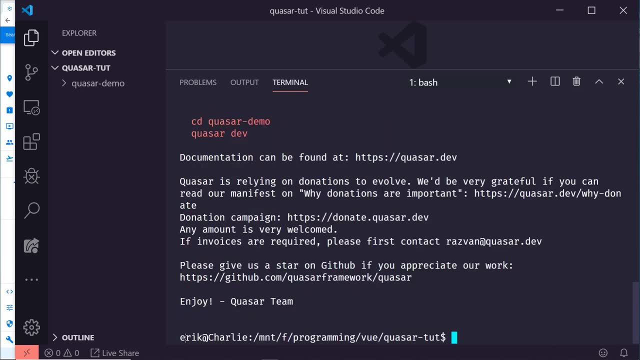 I'll just use yarn And then this will just take a few months and it's going to create the directory structure for us And we'll take a look. Cool, All right. So it looks like everything is up and running and stalled, so we can go to change directory. Quasar demo and then one Quasar dash depth. 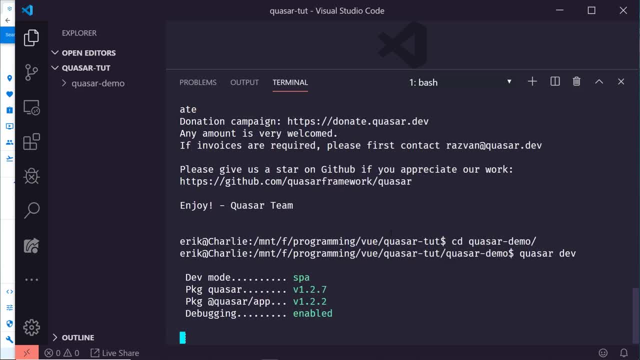 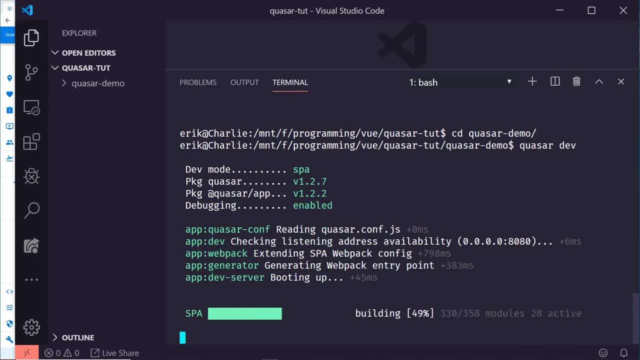 Cause I already have the Quasar CLI installed and that'll go ahead and just run everything up And it actually- I believe it opens up a Chrome window or your web browser window, depends on what your default is- And it should open up here in one second. 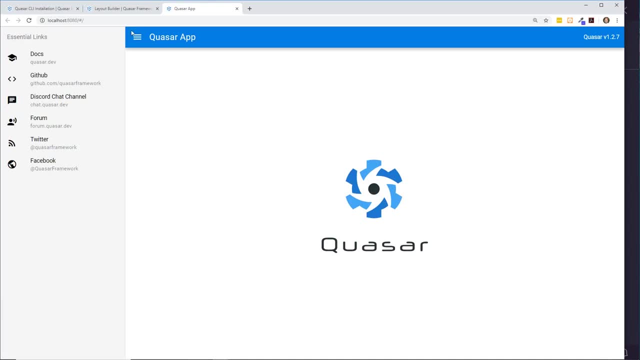 Cool, Here it is. So this is what you get out of the box- Cool, And it just kind of gives you a links here to the demo, the documents, the discord channel. So if you need some help, jump on discord channel forums Twitter. 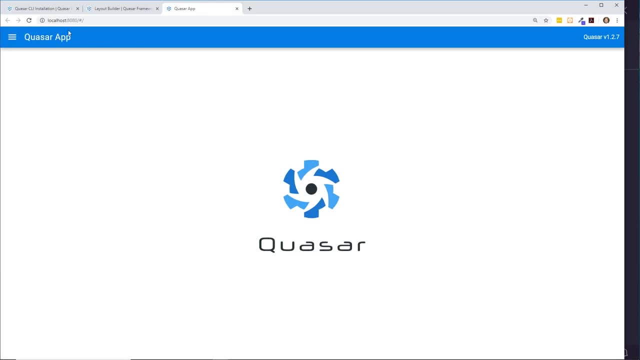 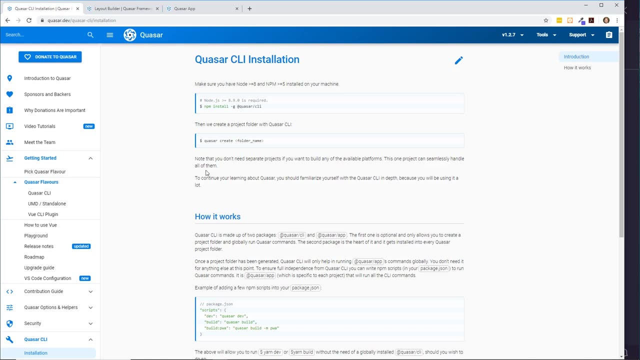 I mean, there's so many things that Quasar is is doing and it has this little uh option here to close and open it. So if you look at the Quasar CLI installation, that's um it mentions to you about how to install it. 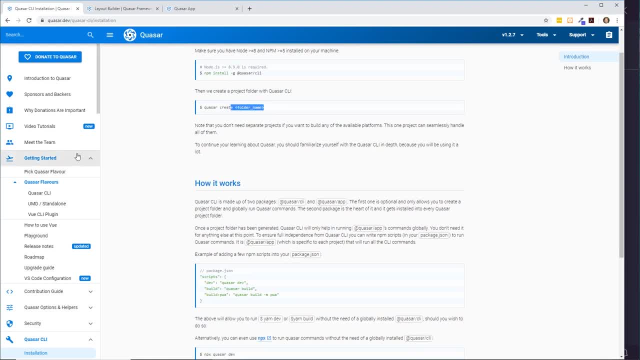 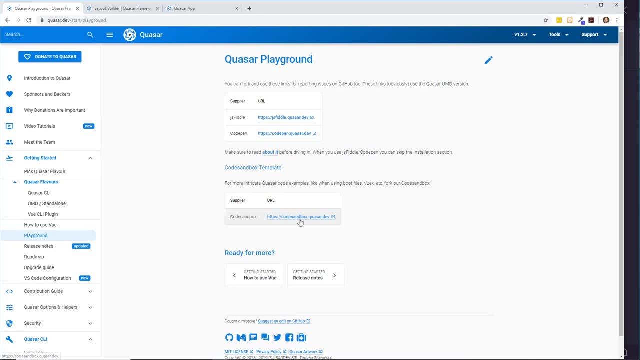 And I just want to mention one thing too: If you go into the playground Under getting started, So if you want to follow along at home, I highly recommend click on the code sandbox link, which I should make everything a little bit bigger. 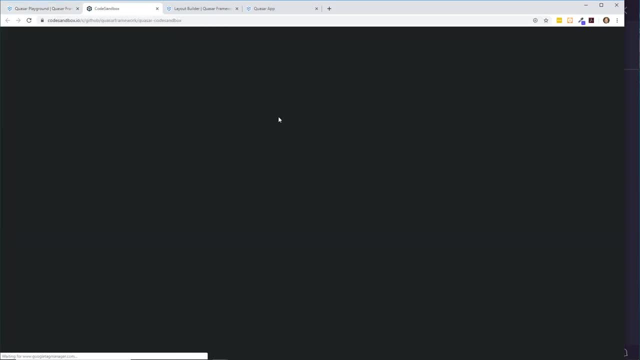 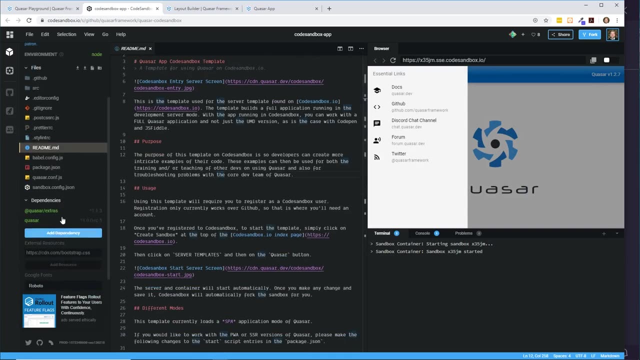 Yeah, Click on the code sandbox link and that'll open up the code sandbox and it has the full ID there. You can then go in and just play around with it, And so that way you don't have to install the CLI and install everything, just to kind of follow along with this demo that I'm doing today. 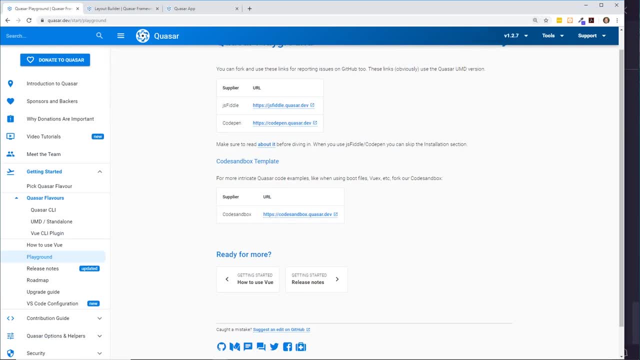 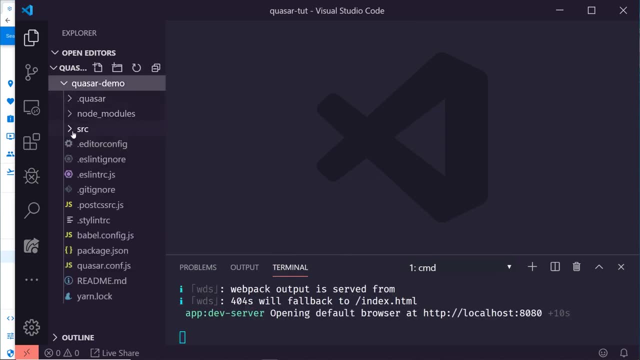 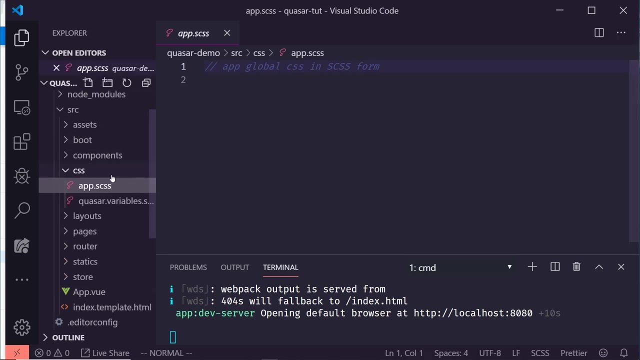 So, yeah, make sure you, you know, check, Check out the code sandbox. So let's take a look at our directory that it created. So here's the Quasar demo. So you see, here I have a source folder and in the source folder I have our CSS, which we chose: uh, S D S CSS. 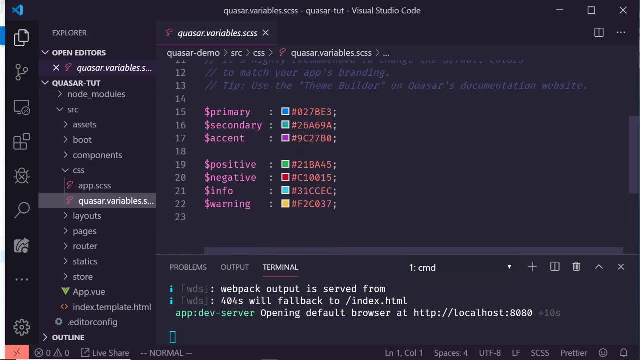 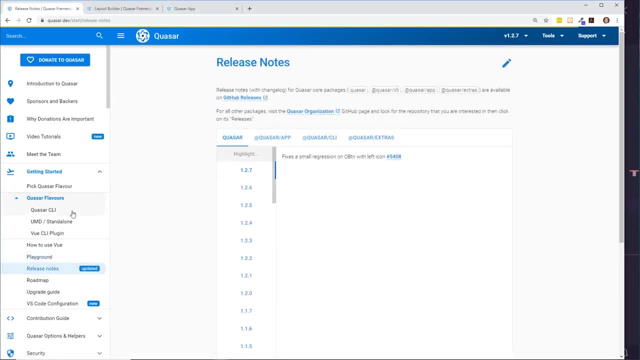 And here is our variable. So this is kind of the look and feel that comes out of the box. So here's the primary secondary accent: positive, negative info warning. A good thing I like to do Is if you go Into the official documentation and go into styles and a style and identity, there's actually a theme builder. 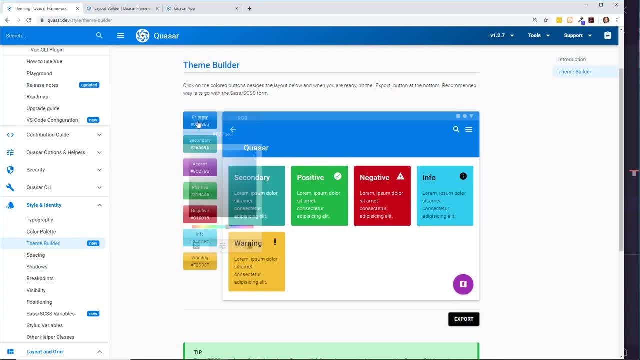 So if you want to kind of add in your own look, looks and feels, you can change the primary, change it to gray. Maybe you want the secondary color, uh, to look, you know, maybe you want it more red. So once you kind of figure out, like the color scheme that you want, with all your positives- cause you'll be, you'll. 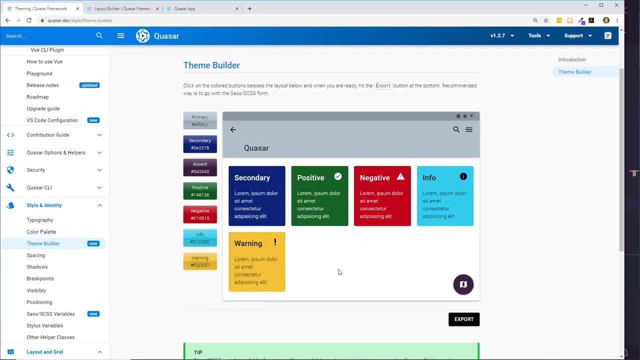 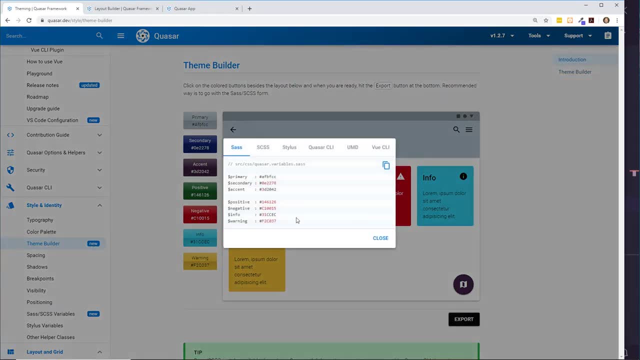 Be using. any time you use, um the CSS classes or you create, you add your own buttons, you'll have these color schemes Um you click export here and it gives you all the number. uh, all the hex for it. 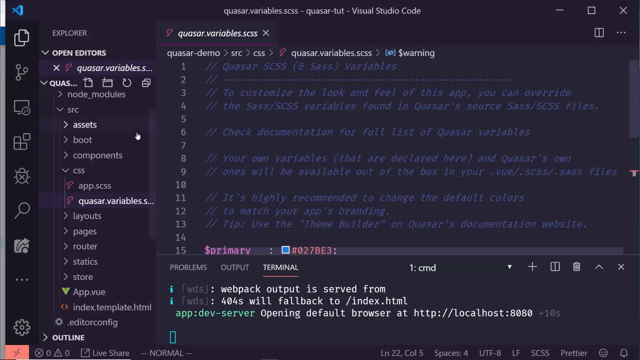 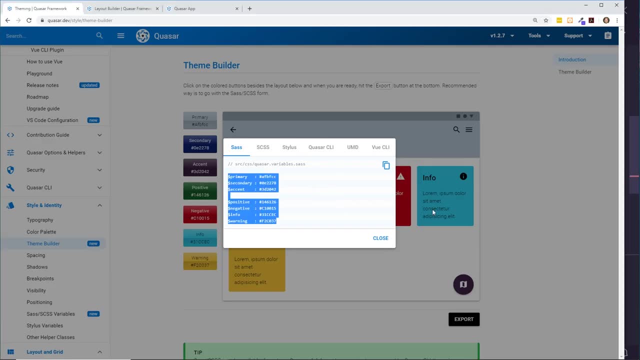 So you can just copy and paste this directly in to your CSS Quasar variables. So you do it, basically overwrite these with the ones you get from your theme builder, And that's what I always like to do. As soon as I start, I always change the default look, uh, the default colors. 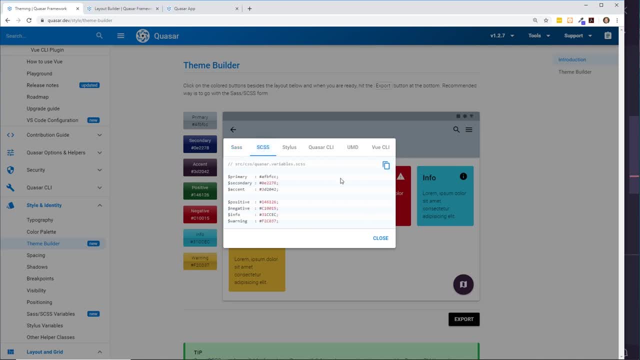 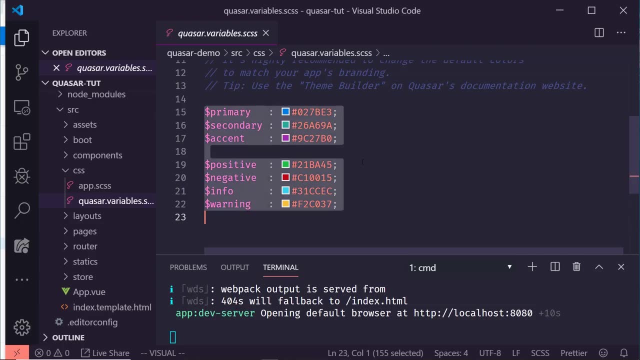 Cause I want my own Colors and, yeah, I just grab them out of here. um, which would be this. that's the SS. I'm not gonna do that right now, but that's something you I would recommend to start off with. 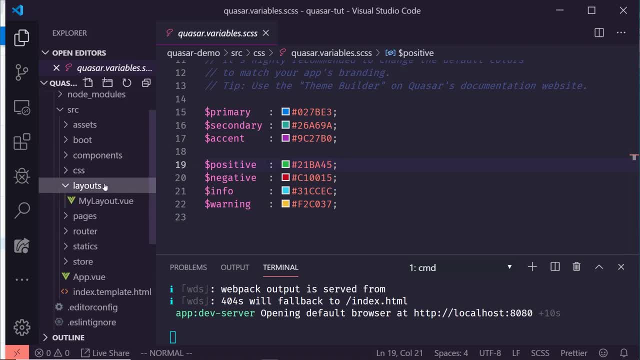 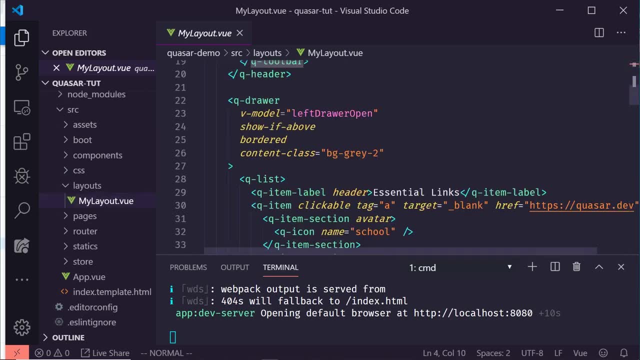 Then, uh, this is where you usually keep your components and the components. Um, this has a default layout. Um, this is the layout here with the toolbar that we had at the top the drawer. That's the word I was looking for earlier. 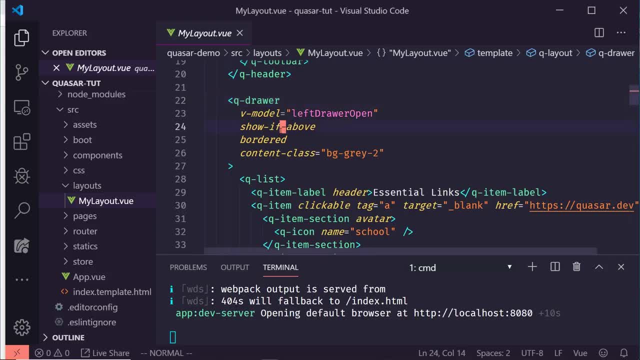 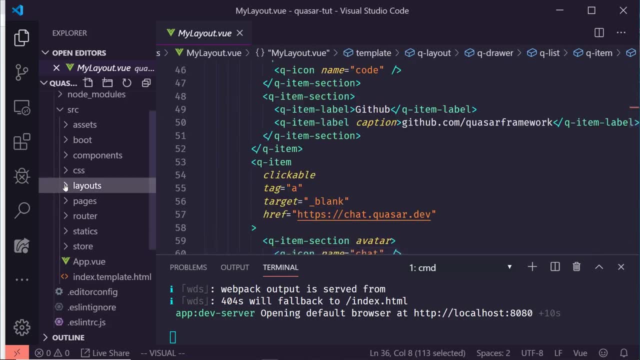 Like: this is the drawer to open, close it And, uh, you have this Q List. So there's a bunch of different custom components that are built in. Now, if you look at the um, we'll kind of skip forward here. 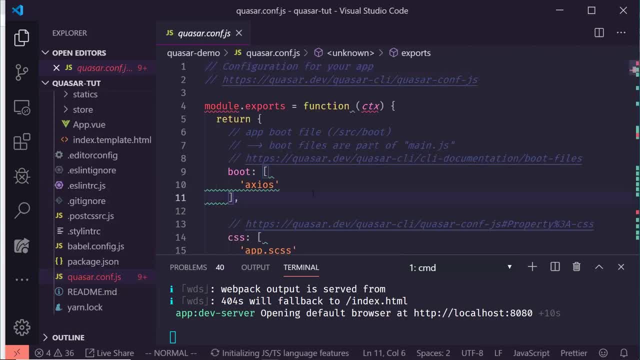 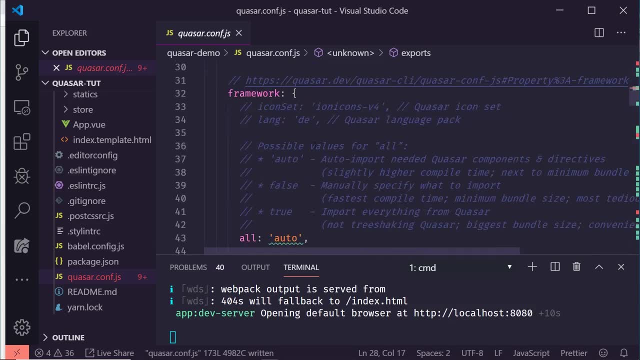 If you look at the Quasar conf dot JS, this is the default um look and feel of it And let me see here If I have prettier. it actually tells me um we might get these squiggly lines. 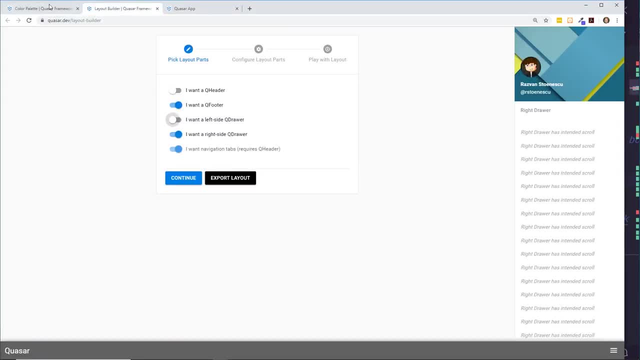 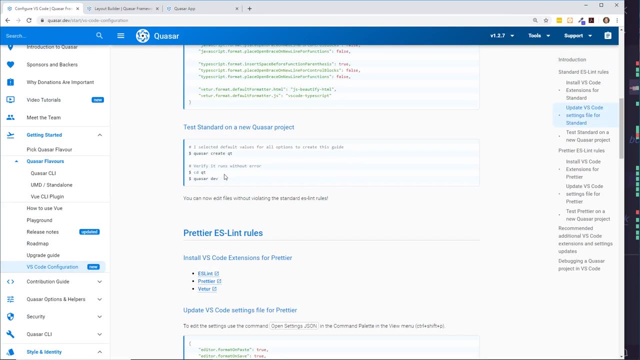 Cause I'm using visual studio code. actually before this demo I didn't change it. If you go into VS configuration And you look at the standard ESLint rules, it tells you what you should turn on If you use prettier ESLint rules and what plugins to install. I didn't do this. 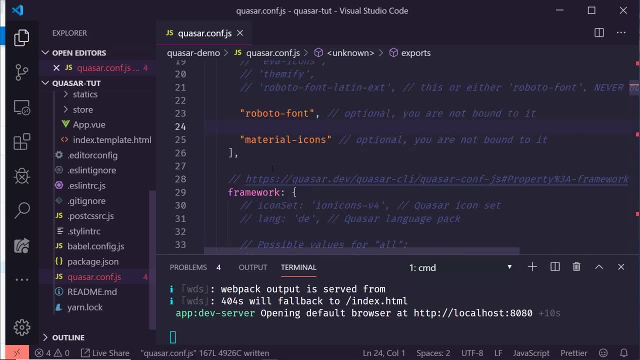 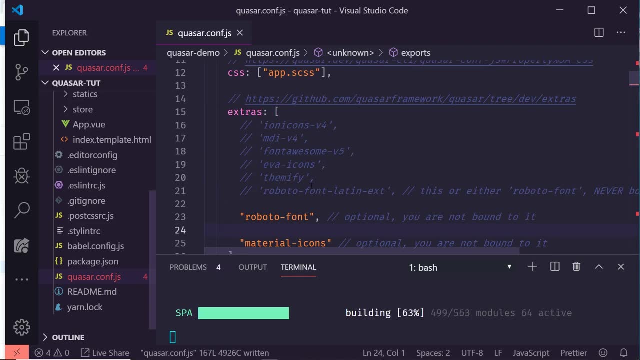 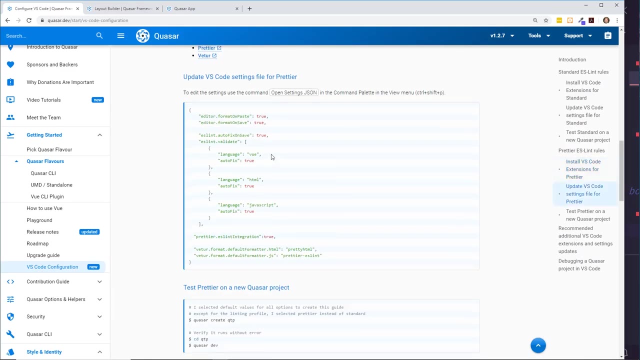 So we might have um. okay, there it goes. Actually, I have it defaults to um single quotes, but I have my prettier set up for double quotes. So when I saved it um, it auto formatted everything for me. but if I wanted to to set up the right way, I would probably go in here. 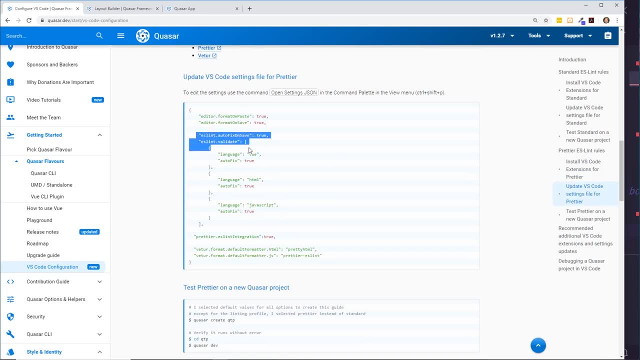 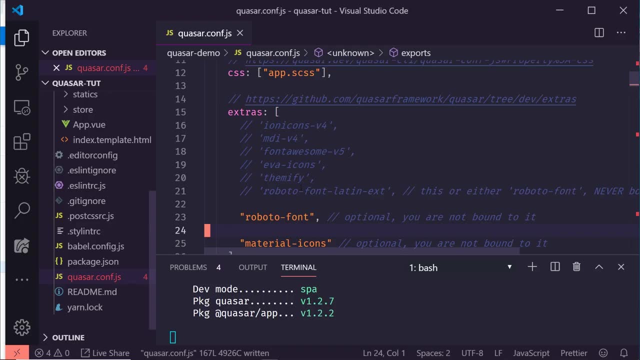 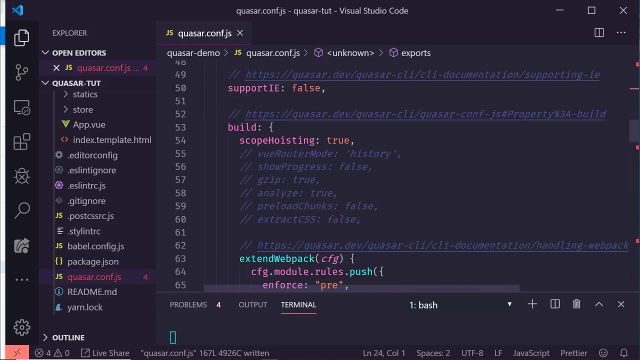 And and do this. So this is the way to set up, like the auto fix on save um language prettier, ESLint default formatter. Anyways, uh, one thing to look for inside this Quasar conf file. If you look at the top here, let's see here: 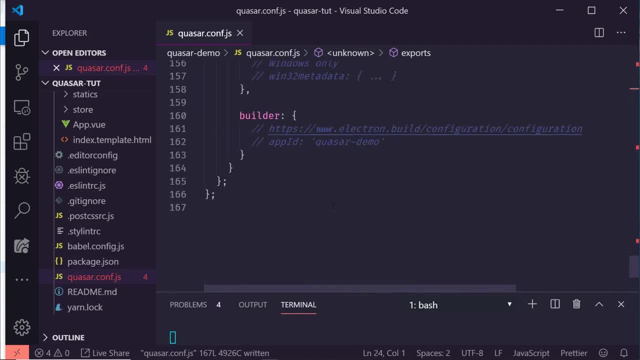 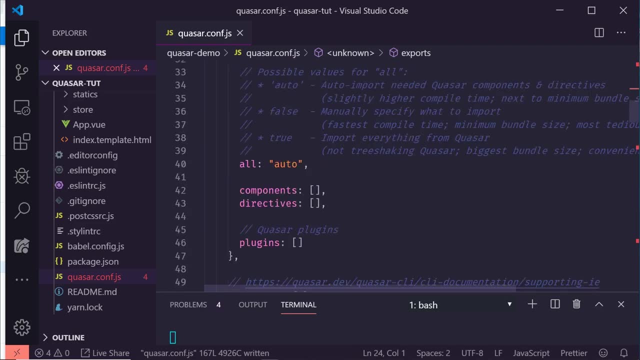 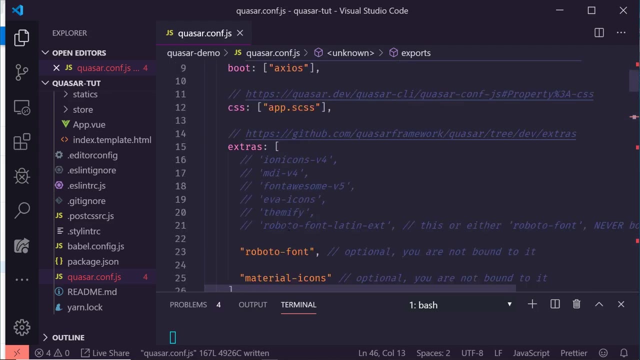 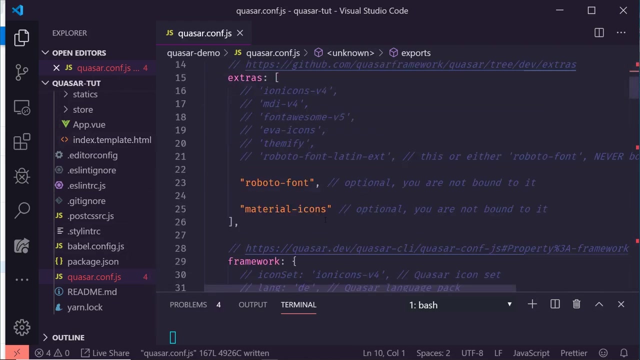 If we look in, I think there is a section For what we have installed yet- components, directives, plugins. So if we wanted to have um certain plugins or directives, we would go ahead and add them inside there, which we could do um which we'll do later. 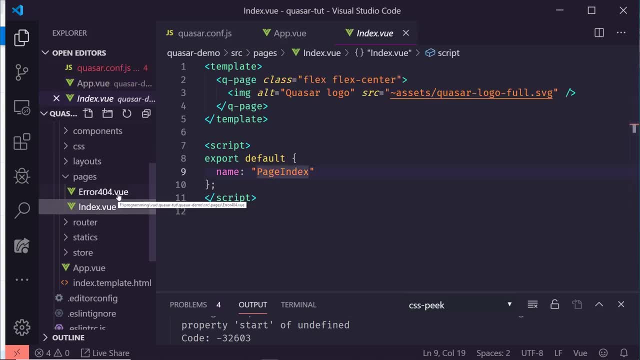 Okay, So we can have these pages here. Pages are basically just normal components that we can have. You can hold a lot of information inside them if you want. It depends on how you want to set up your app. If you go to the router file. 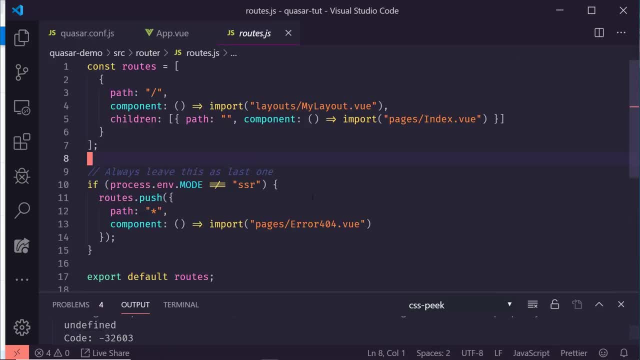 You can see inside the router file, here the these: this is how we set up our routes. Um, so it's pretty normal. This is actually using lazy loaded routes, and you can see here it's the children. So let's say we wanted to create another child, so we can easily do something like this. 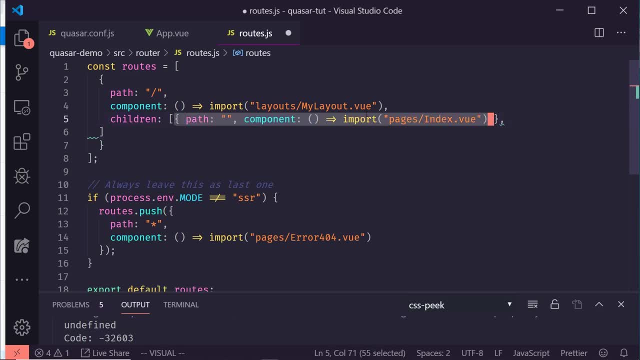 Just grab this, copy it and then, instead of having it path equal there, we'll do path I don't know- Pass Pass, Pass, Pass Pass, Veggies, Veggies, cách, Dark Connect, And we'll just use Objectiveuum slash, web slash eric, and we'll make a pages called 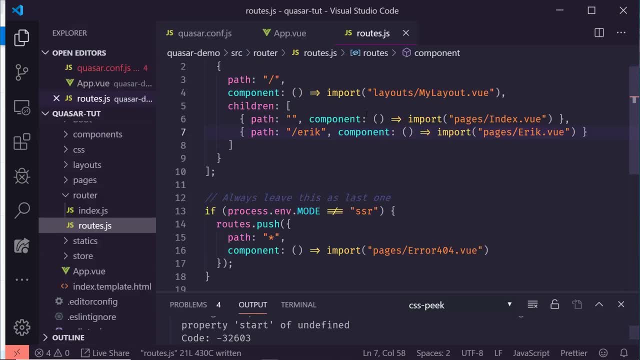 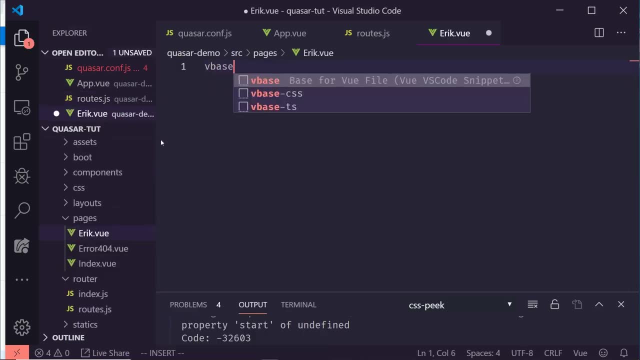 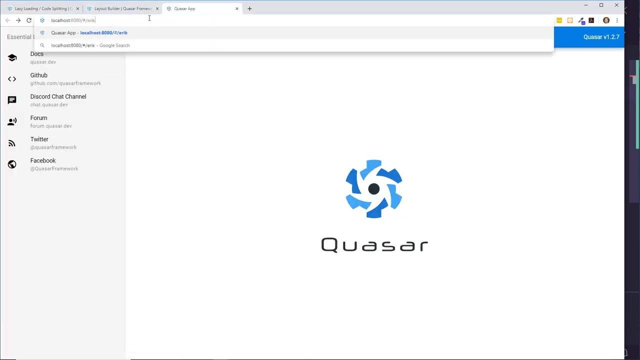 ericview and let's go ahead and create that page. so I'm going to create a new file, ericview, and we'll do a V base here to an H3.. Hello from Eric. We'll save it our quasar framework here, so if we do slash eric there, it is hello from eric, so perfect. 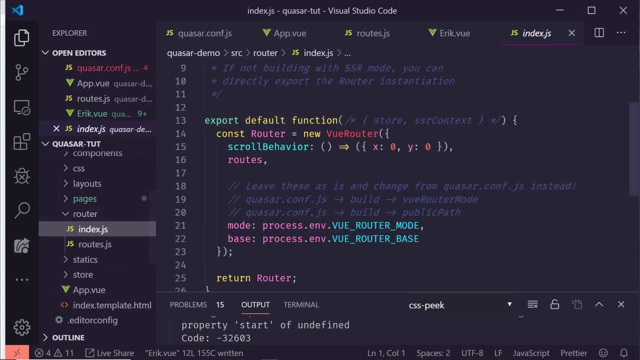 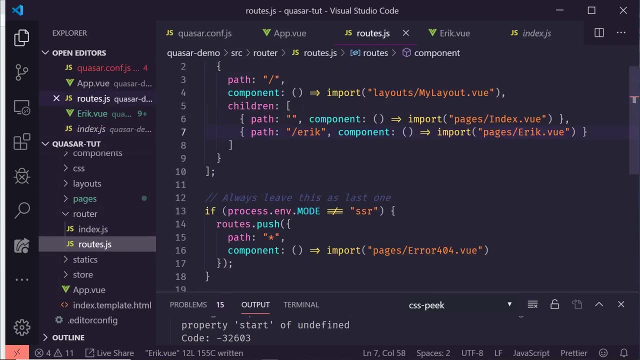 then we can also, like i said, we have our router, which we have this index route, which i wouldn't even change, but if you look at the routes, this is where the routes is, and then we have static files we can add in here, and then i added the vuex store, which it goes ahead and gives you. 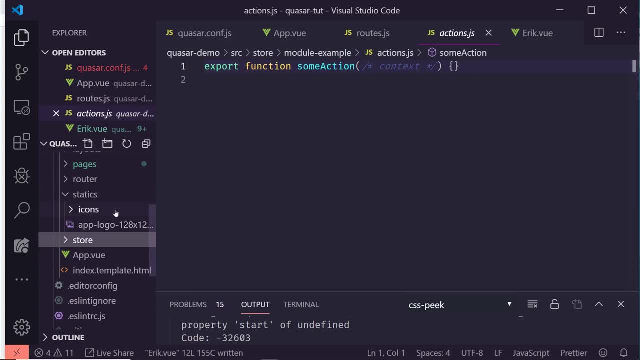 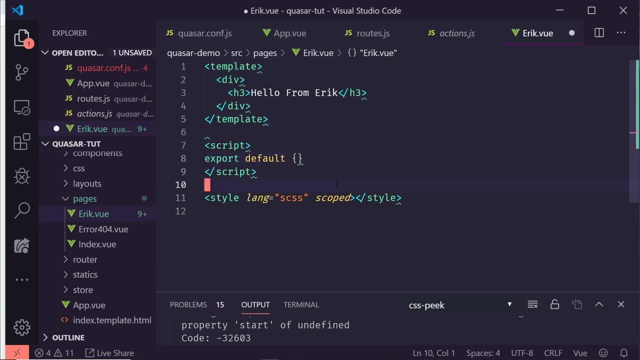 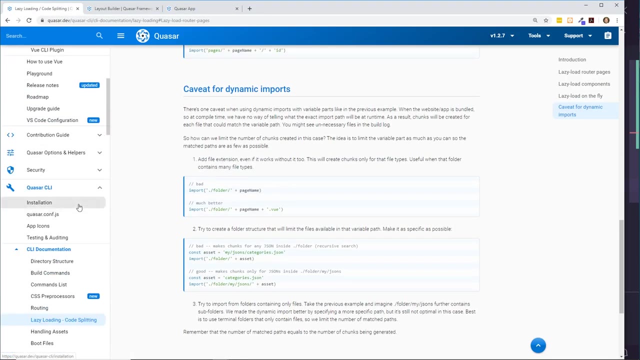 some module examples of how to get modules installed. so we're not going to look at that. so in our pages here, ericview, um, let's see if we can add in some examples from our code here. so i'm just going to add a couple in to take a look at it. so first thing is, we can probably look. 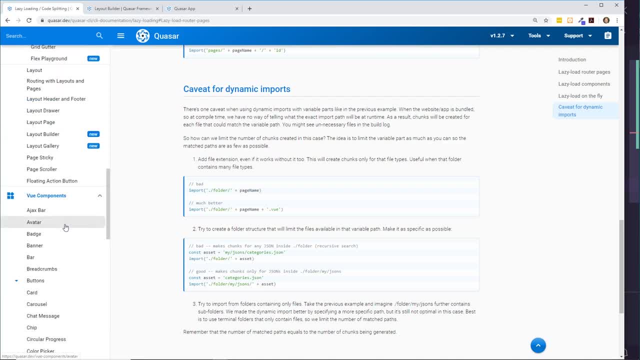 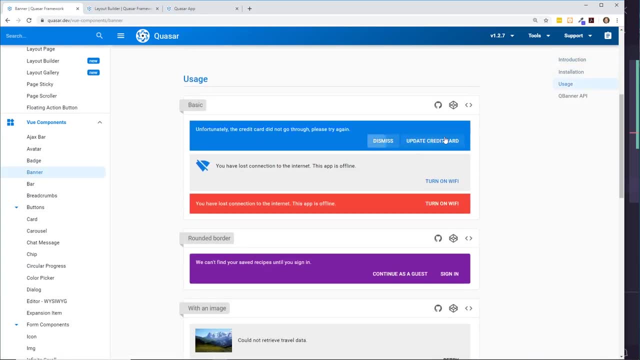 at: uh, let's look at a component. so let's take a look at a banner. so, fortunately, a credit card and i go through dismiss so you can create banners like this. and one thing i like to do when i'm just testing stuff out, i just click here and just 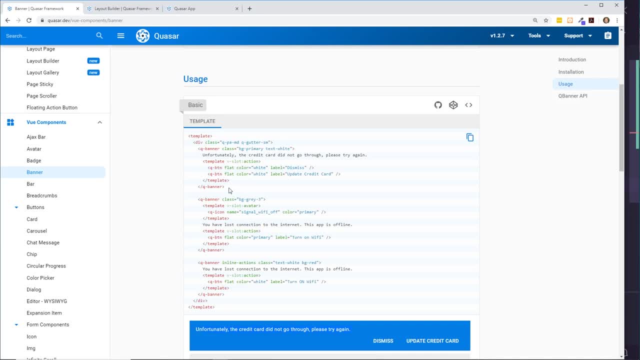 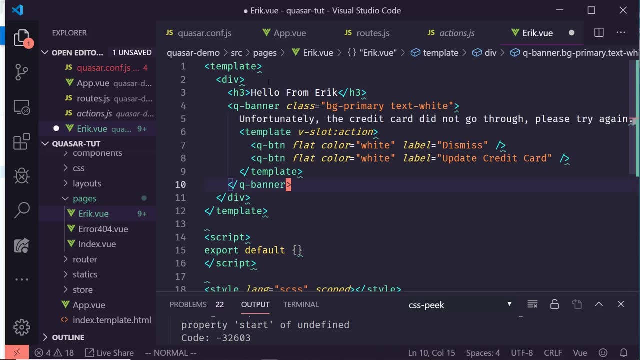 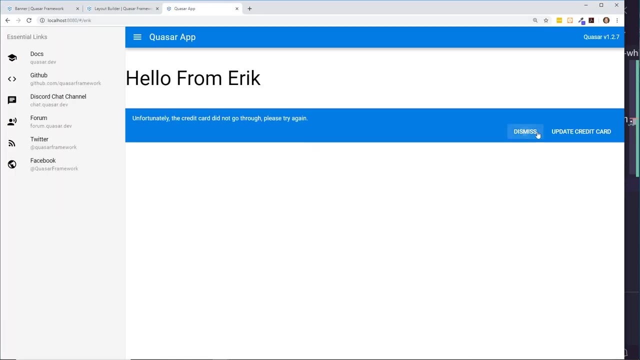 copy and paste some of the code. so, uh, here is a banner right here, so i'm gonna just add it in here and see what happens. so i'm gonna look back your quasar. yeah, here's our banner: dismiss, update credit card, um, and then i'm going to go ahead and create a banner, and then i'm going to go ahead and. 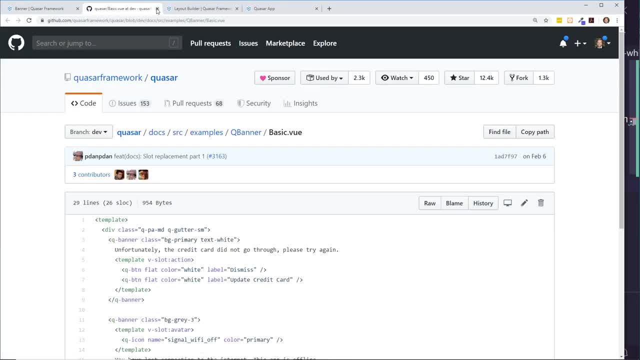 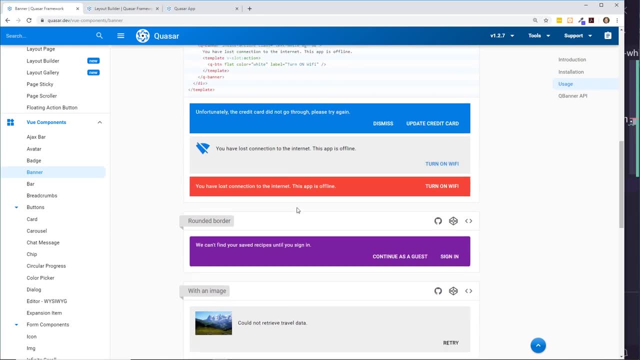 paste some of the code in here. um pretty neat. we can even open it up in github if we want. or look at the code pen of it. um, here's one that says you have lost internet connection. so if you look at all three, i guess i can add all three of them in here. 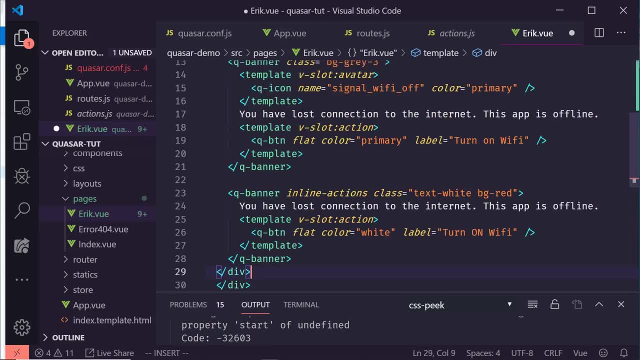 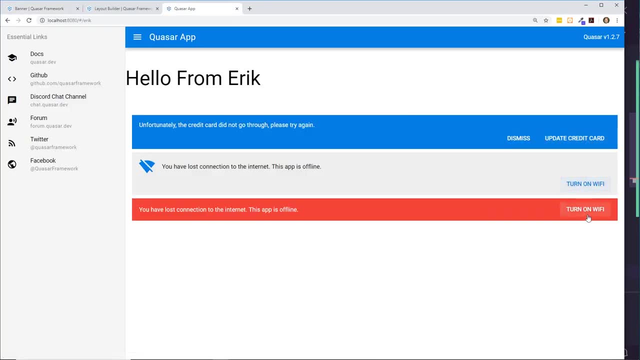 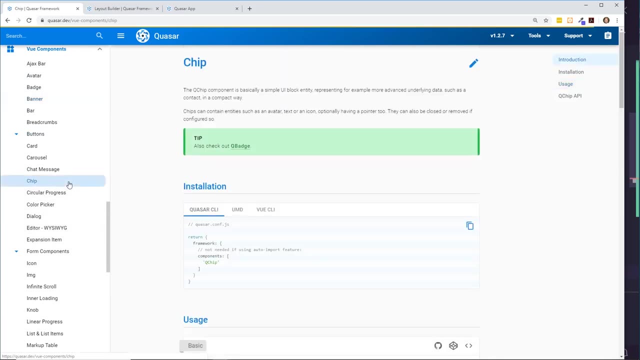 let's take a look here. just delete all three here and i'll save it. yeah, cool. so yeah, it looks exactly like it looks exactly like this, so i'm going to go ahead and paste it in here. so i'm going to go ahead and paste it in here so i can kind of play around with it. 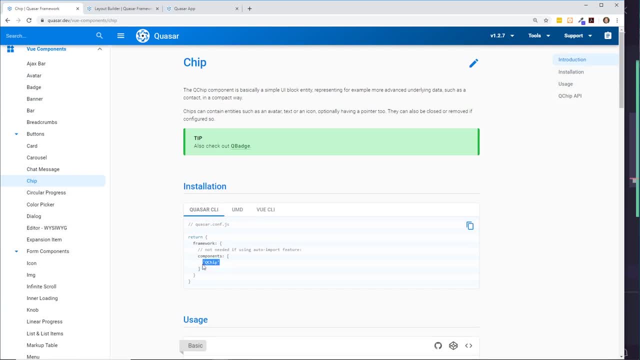 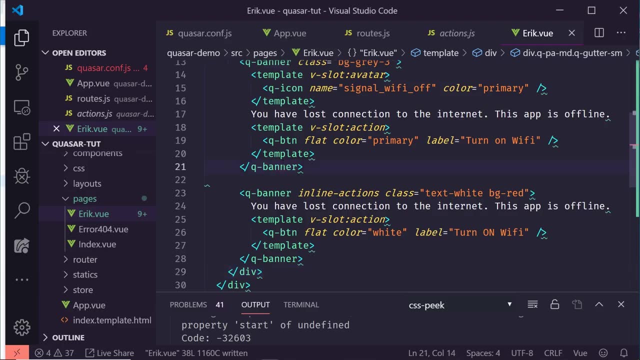 one thing you might need to do. so if you go into like chip here and you look at the installation, sometimes you'll need to actually add the component. so like here says components, qchip. so to do that, what i do is go into that config file, that quasar. 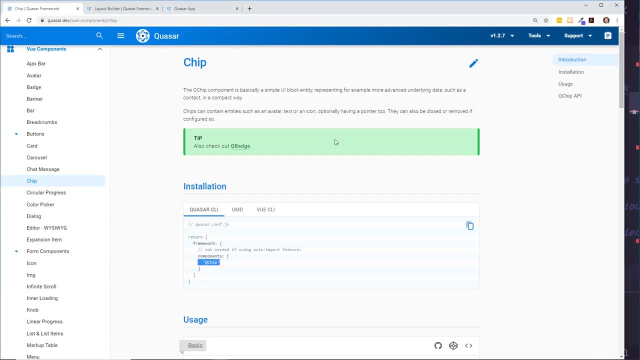 conf and then go into that components again and then you just uh add it in there like this, and then you just uh add it in there, you should be able to use it. so if we go, you should be able to use it. so if we go back to here, 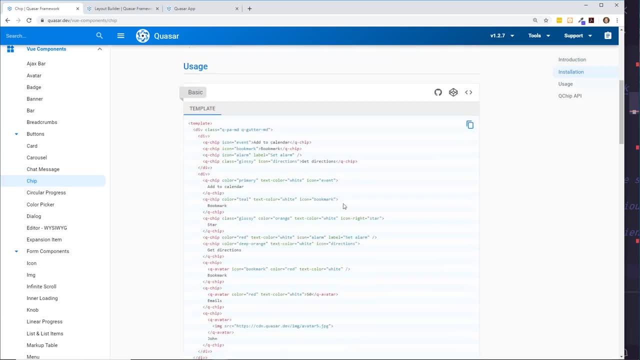 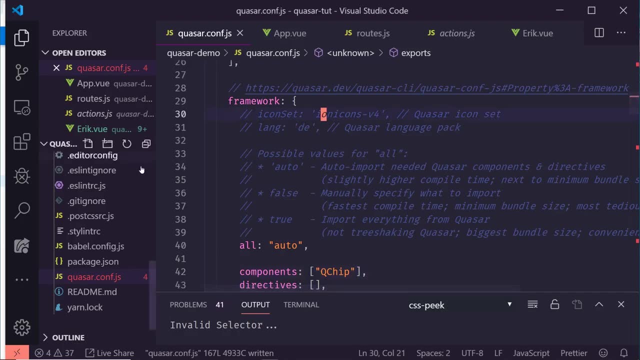 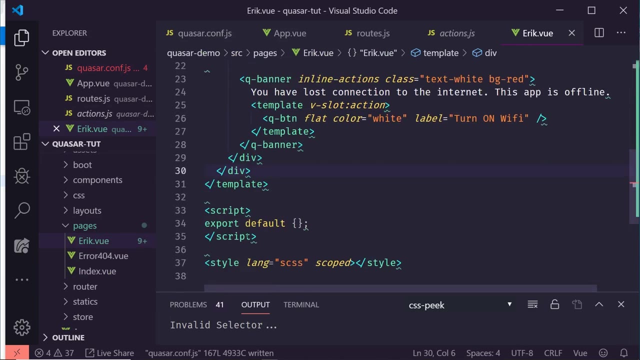 back to here. um, here's a chip example. let's just copy and paste some of the code in here. do that go back to our eric view and, uh, let's just put it right under this one. um, let's do this. um, let's do this. 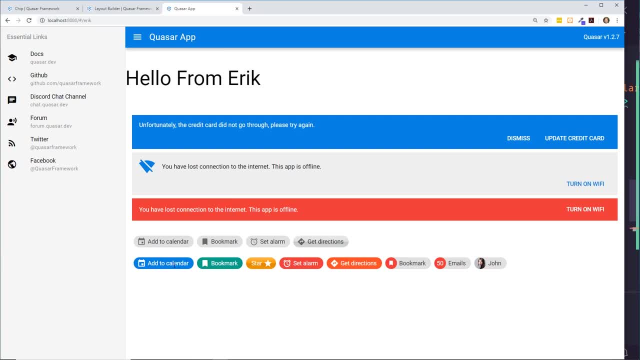 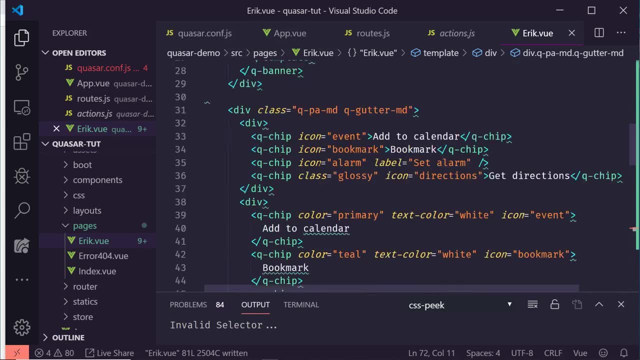 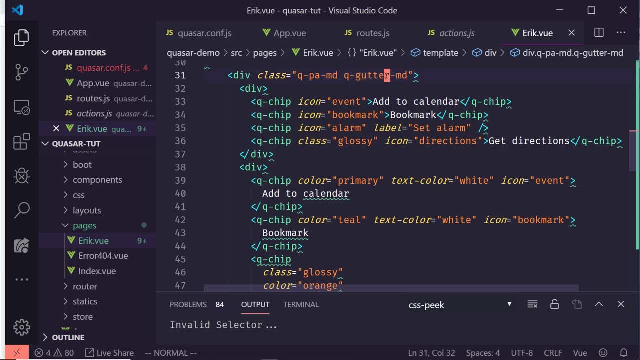 built-in classes to do the layout and formatting. it sort of looks like tailwind css. um, it might even be running some tailwind css underneath, but it has this q dash- that's definitely not tailwind- and then use this q-dash chip to do everything. 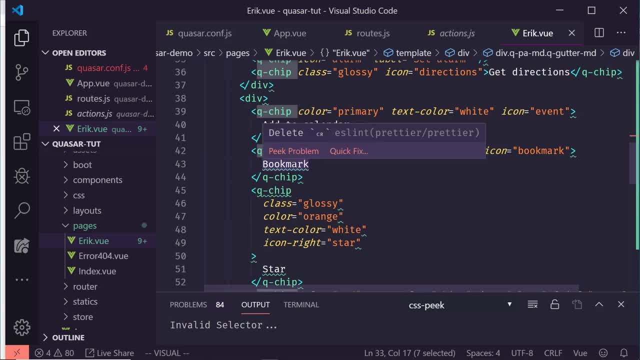 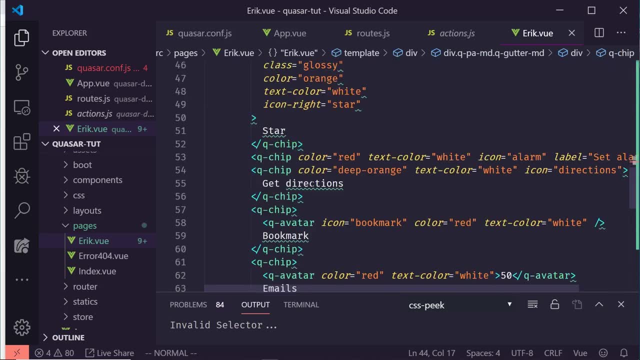 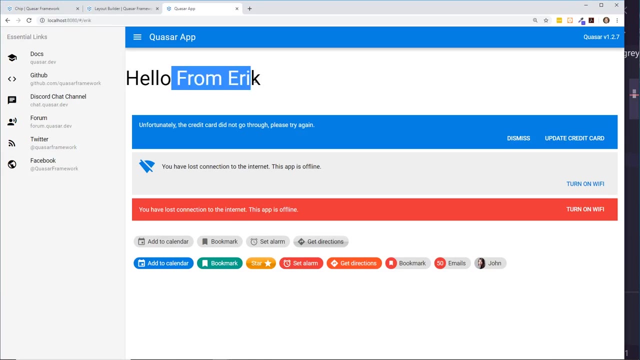 and, by the way, i got a lot of squigging lines here. it's just a a weird issue with um es lint which i'll have to configure in my next video, but for now you can get the idea: directions, bookmarks, emails. okay, so we got all our chips in here. hello from eric. 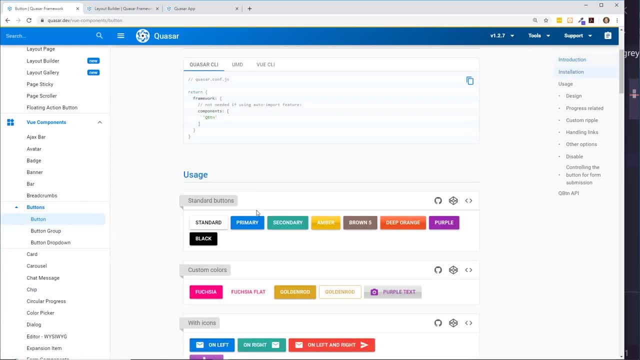 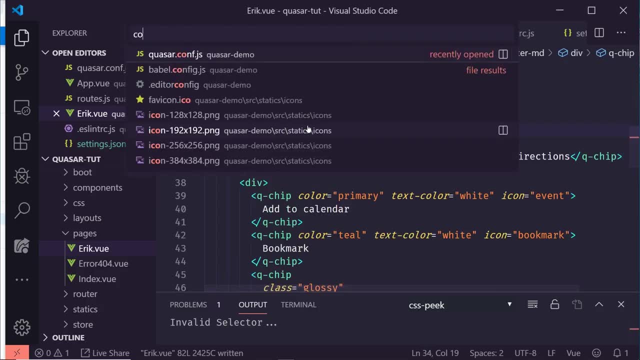 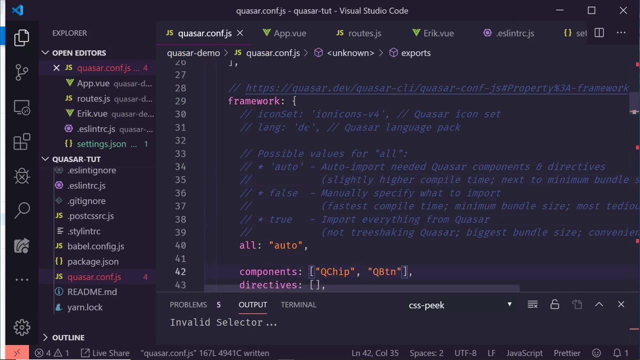 uh, let's take a look at one more. let's take a look at some of the buttons that we can get with it. once again, make sure i have the q button, um, installed here. so i'll go back to my comp file and i'll add the chips. i'll add in q button and then i'll just try out some of these buttons here. 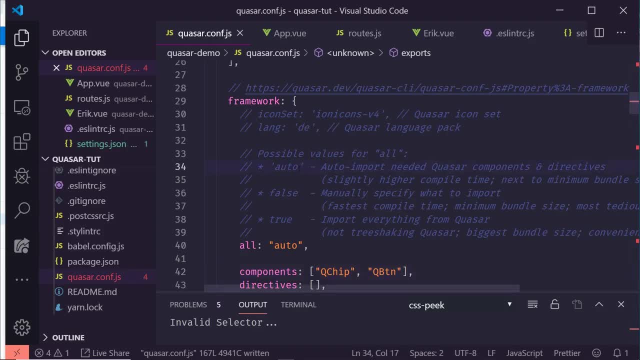 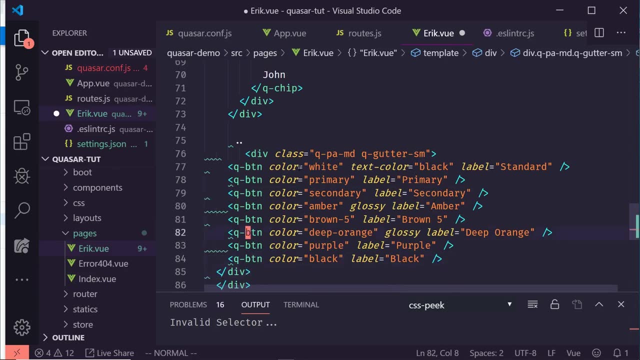 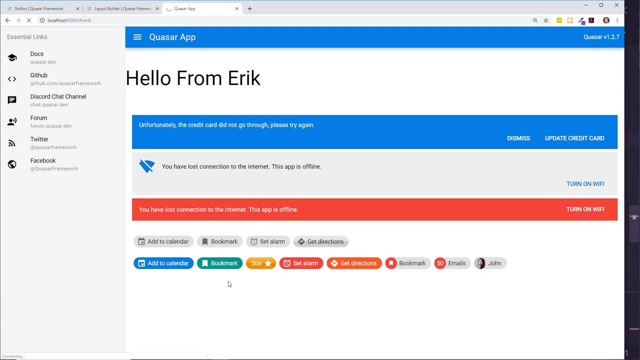 this is where the colors come in mind that we had set up earlier. so we'll go back to my ericview and i can just paste them right here, and if i take a look here- now- i have fit and upstairs- you'll see where this code has fallen down. 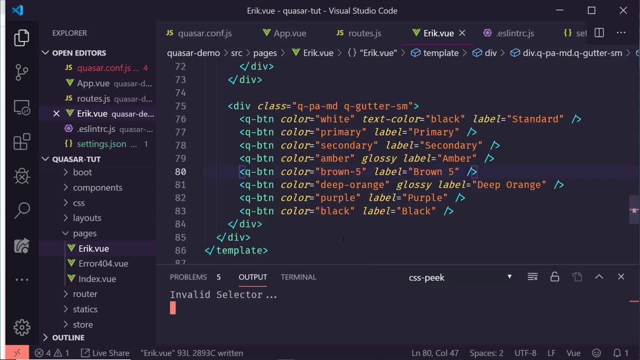 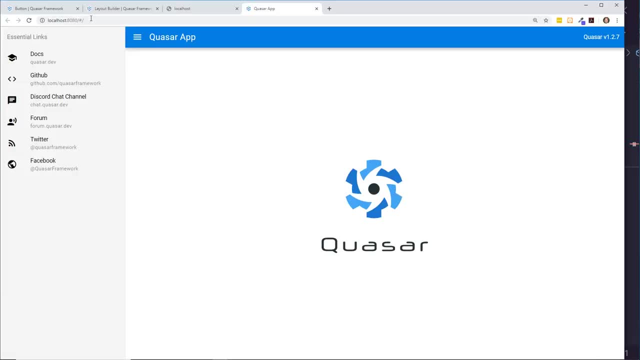 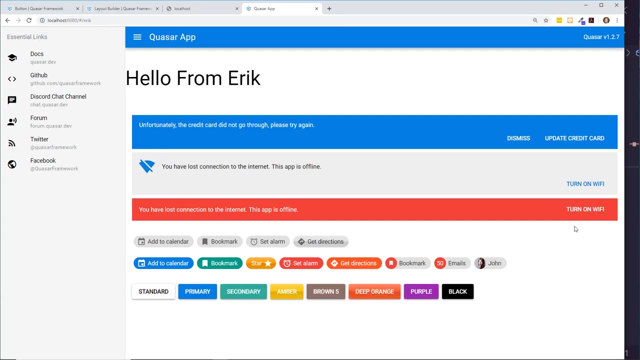 let's continue. it gives me an error. might be. let's see what it's doing: oops, that can't be loaded. let's see here: invalid selector. let's take a look what we are missing here: q button. we'll just ctrl c it and restart it. okay, i actually just stopped and restarted the server. 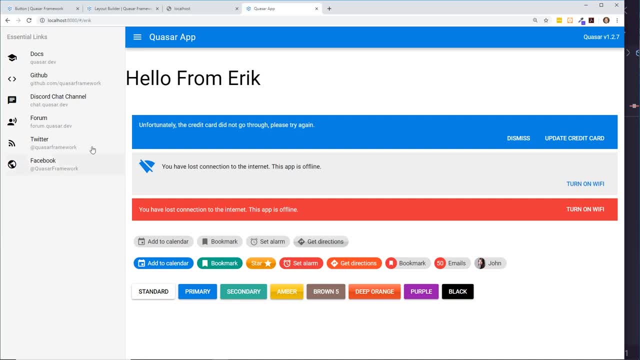 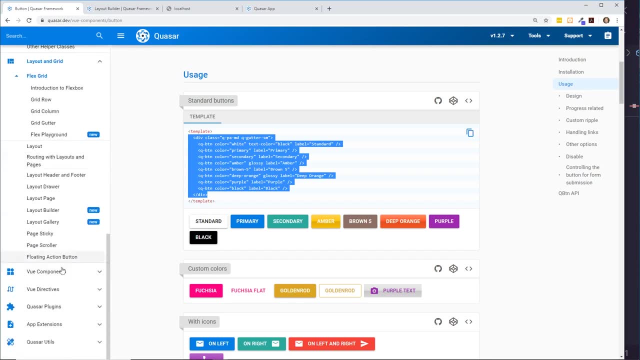 we're going to end it here, but i'm going to show you real quickly one thing you can do. if you look at the official documentation, you scroll all the way to the bottom. you can actually let me see here- i believe it's actually not at the bottom- when we're quasar cli deploying. here it is, so you can. 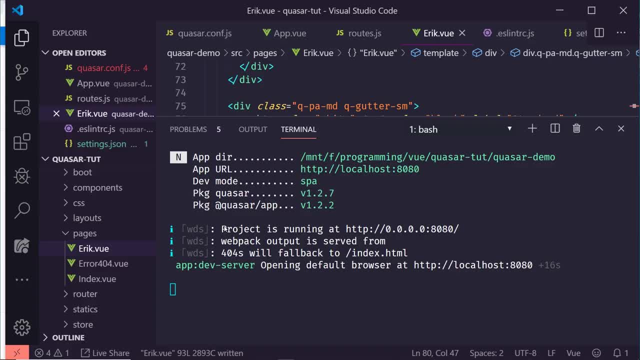 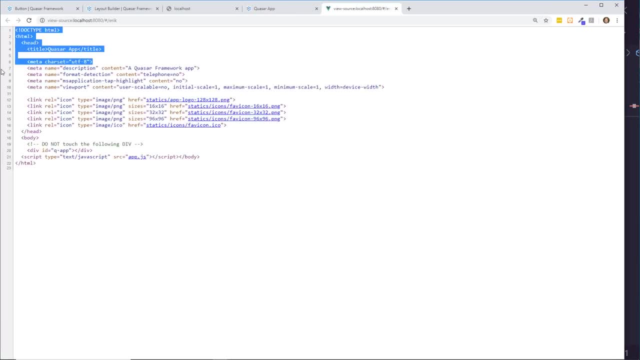 deploy as a spa. so when we did quasarposdev, we're just running it as a single page application and one way you can tell. so if i look at this view source here, i just have this normal html and then i have this div idq app and this is where it's getting bootstrapped, all in the source it's. 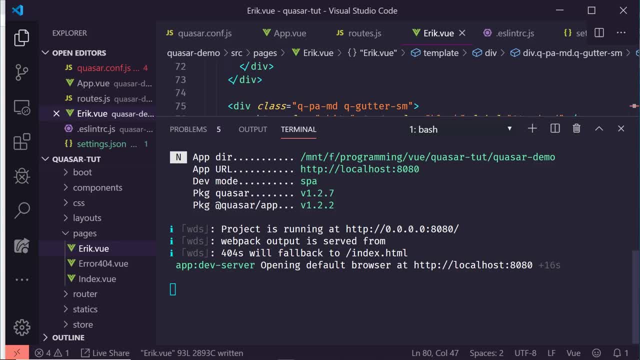 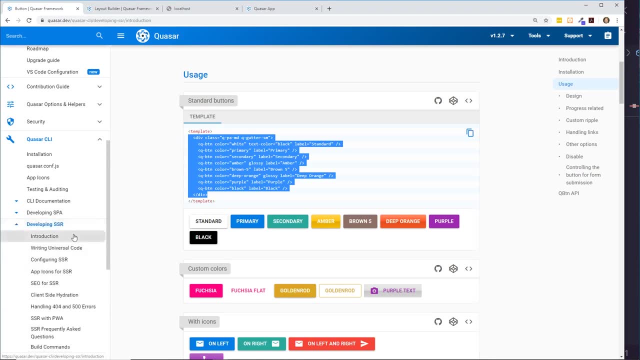 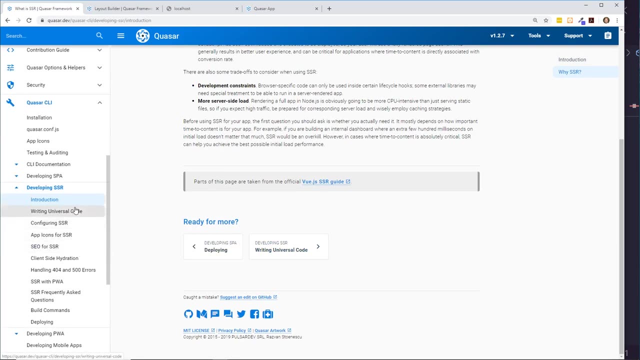 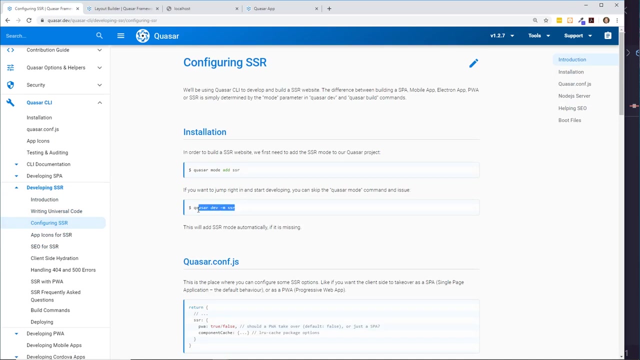 running the javascript and adding everything. but if we wanted to run it, uh, differently, we can look at the official documentation. and if you go to developing ssr- that's a single server-side rendered- you can actually deploy it using ssr, so configuring it. so, essentially, if we just want to test it, we can just do quasar dev, dash m dash. 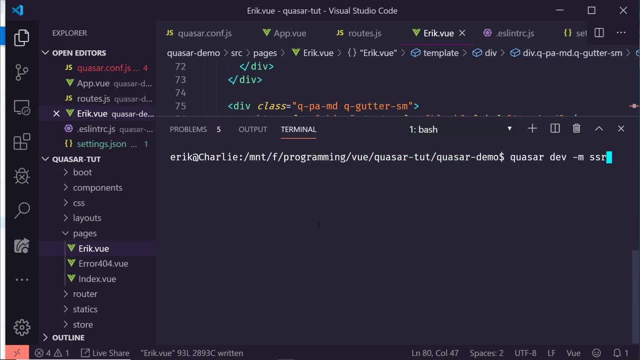 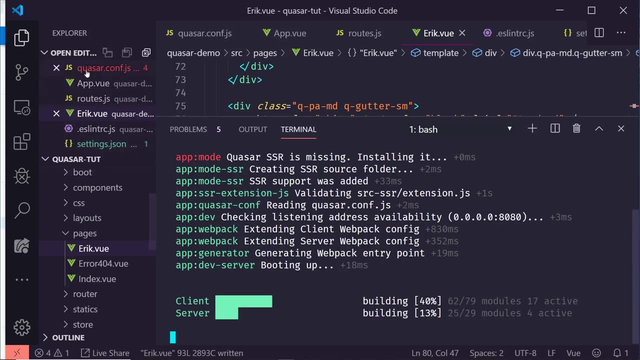 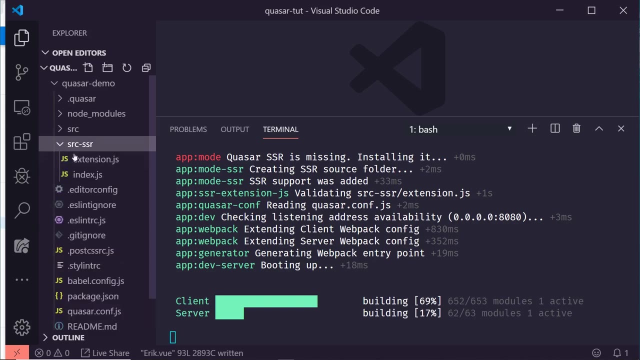 ssr. so if i clear this and i run it now, it's going to run it in ssr mode and it's going to do everything for us and it's actually if you look over here. i'll close these. um, it creates a new ssr source folder where it kind of has some configuration inside of it and see, now it's. 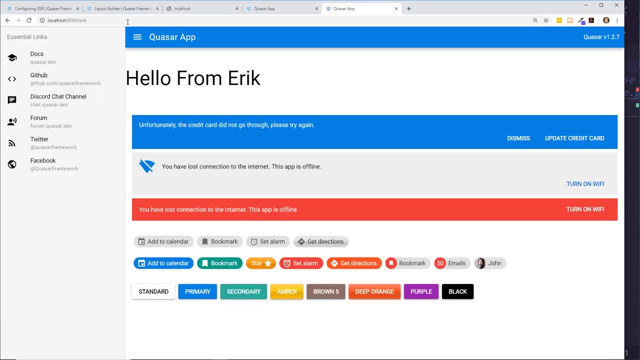 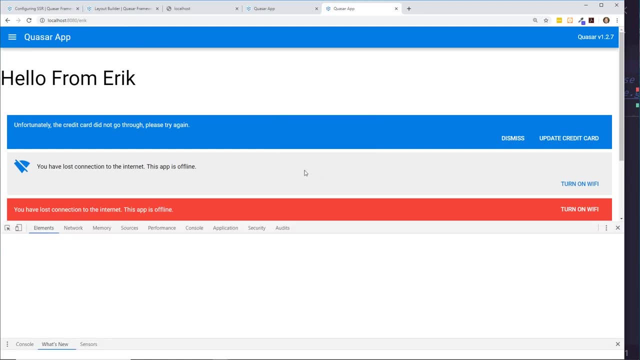 opened in ssr mode and it's going to run it in ssr mode and it's going to run it in ssr mode, which, if i go to eric here, here's the uh information. this is just the different components we were testing out. if you look at inspect here- actually view source- you can see. 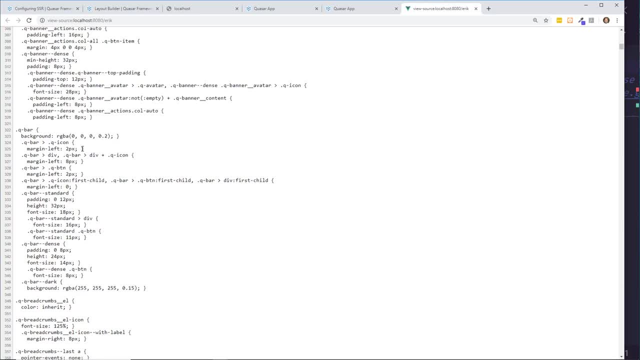 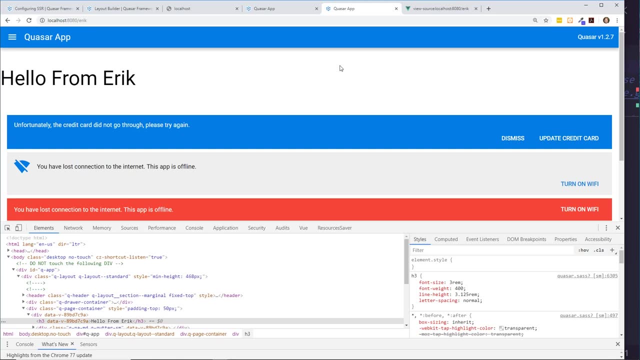 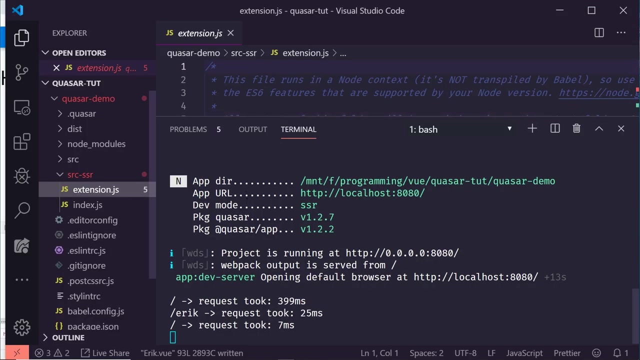 now it has all the details. so basically it it sent this all down on the initial load, so it's much quicker because it's it has all that server-side rendered goodness built right in. so that's one of the cool things about using quasar is that just with one simple command we can go ahead and set up for ssr mode and we could 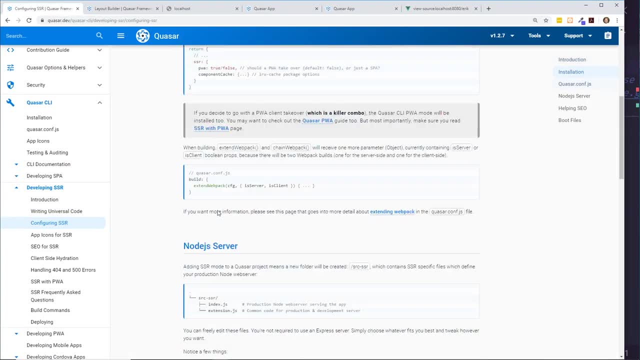 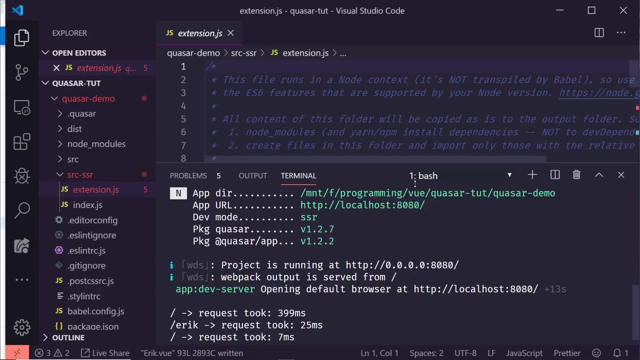 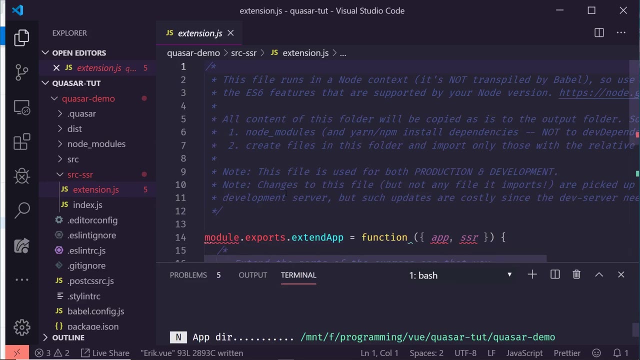 even if we wanted to. that was just configuring it, but we could just build it for ssr mode as well if we like want to do that. so that's all i'm going to show you today. that was just a few components. i want to see and hear from you guys what, um, tell me what sort of components you want me to do in. 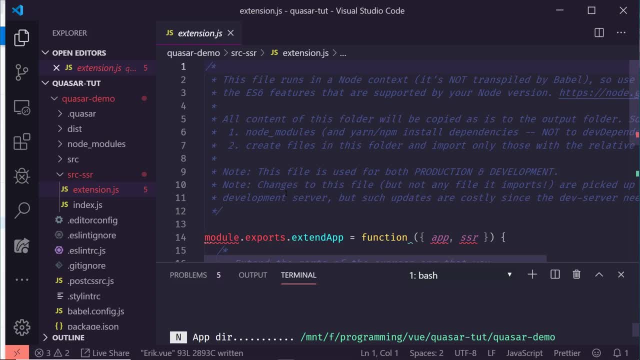 the future. what features are you guys interested in? and i'll see you in the next video. i'll do, uh, my next video. i'll create a small little app using quasar and then i'll show you how i can connect to like a third-party api and then display the information in like a table or 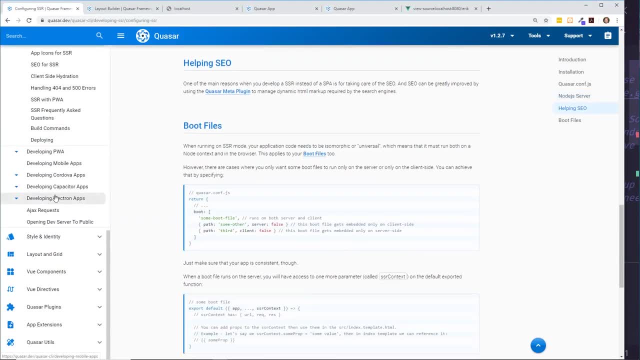 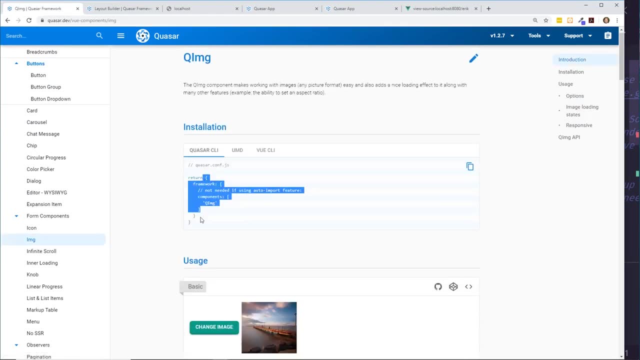 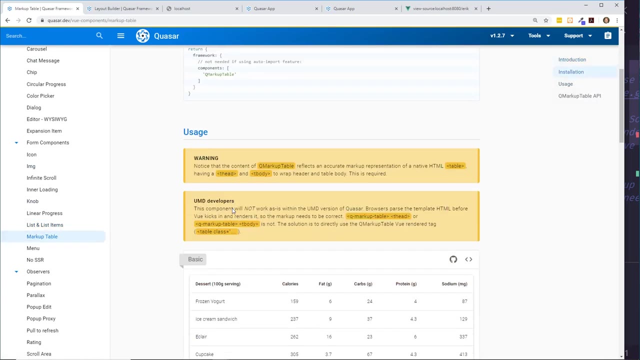 or using some one of these quasar components, because there are so many, maybe we even use a directive to like to have a carousel. they have their own image so you can set your images. they have like lists so you can easily set different lists. they have a markup table. so yeah, so there's. 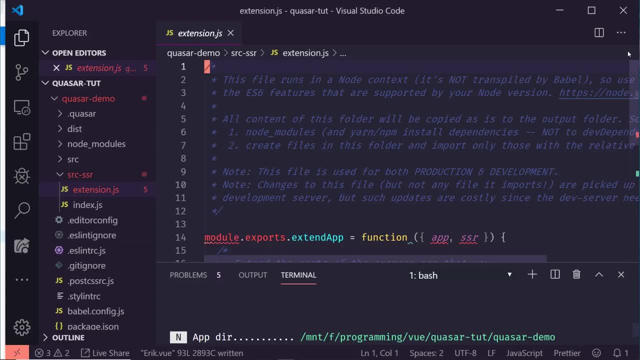 so many different things. i'd love to hear what you guys want me to do next. um, if not, stay tuned and i will go ahead and show you guys a little bit more in the next video. thanks,